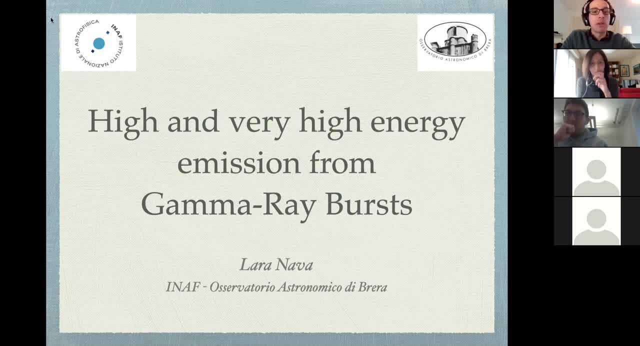 bursts. Just a reminder. questions are welcome during the talk. You can either raise your hand or write them in the chat box and I'll read them over to Lara. All right, Lara, if please go ahead? Thank you, Okay, thank you. Thank you for the introduction. 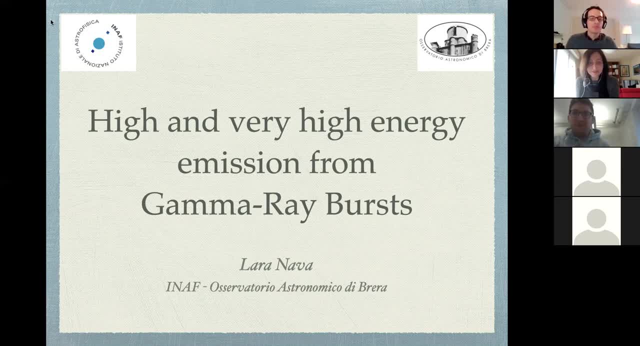 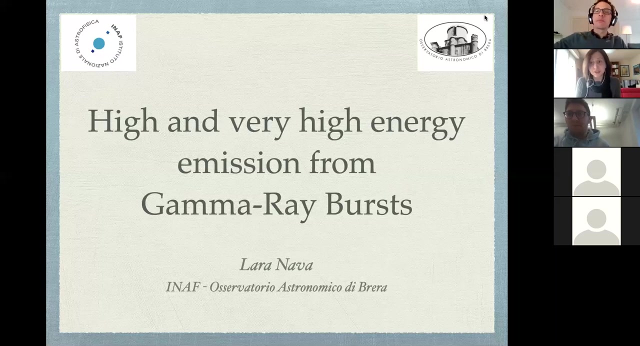 Thank you, Thank you, Thank you And thank you for the invitation, And so let's start. I will first give a general overview of the gamma-ray burst phenomenon- So I'm assuming that most of you are not familiar at all with gamma-ray burst- and then I will pose for questions on this first part of the. 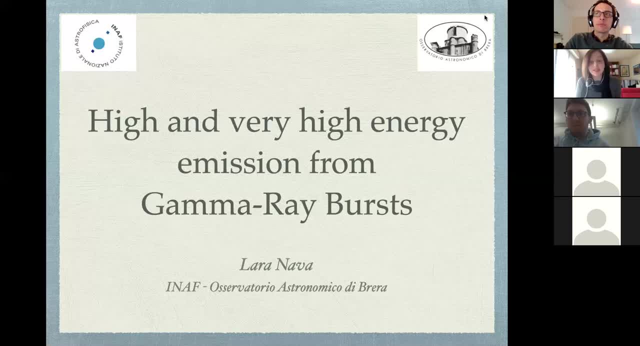 talk And then, in the second part, I will focus on high energy emission from gamma-ray burst- Thank you, energy emission from gamma-ray bursts and, in particular, on the recent discovery that gamma-ray bursts are TV emitters. So let's start. 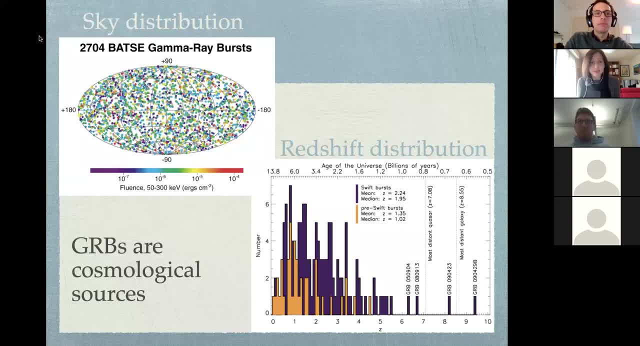 So gamma-ray bursts are cosmological sources. so here you can see the distribution in the sky that is isotropic. so this was the first clue that gamma-ray bursts are extra galactic sources. and since 1997, when the optical counterpart was discovered, we can measure the red shift. 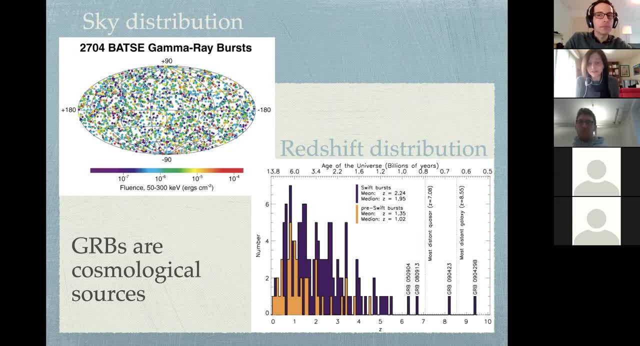 for most of gamma-ray bursts from the after-glow optical emission or from the identification of the host galaxy. So this is the red shift distribution of gamma-ray bursts. Colors just refer to gamma-ray bursts detected before Swift or a after SWIFT in the SWIFT era, so since 2004.. 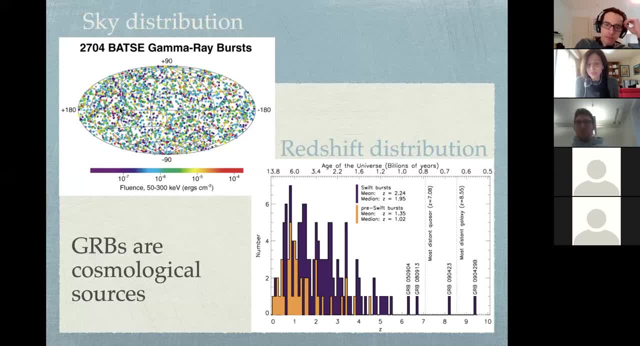 So the mean redshift is around two, but, as you can see, several gamma-reverse have been detected also at quite high redshift, so about four, And we also have a few gamma-reverse detected at redshift larger than six, And the record holder is currently this gamma-reverse here. 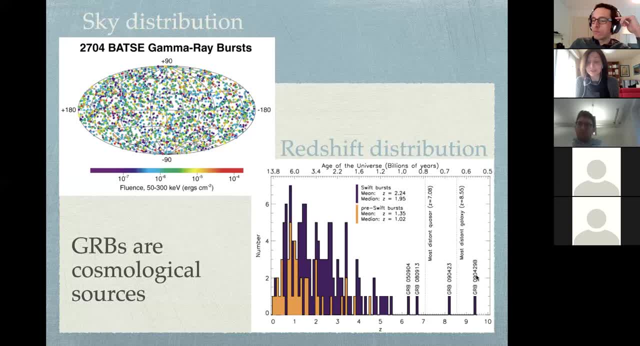 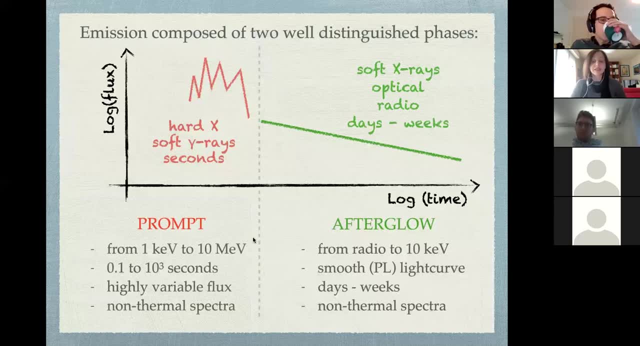 or 904.29b detected at redshift 9.3.. So the emission in gamma-reverse has two well-separated phases, the prompt and the afterrule. So the prompt emission here in red is detected in the soft gamma-reverse band, hard X-ray. 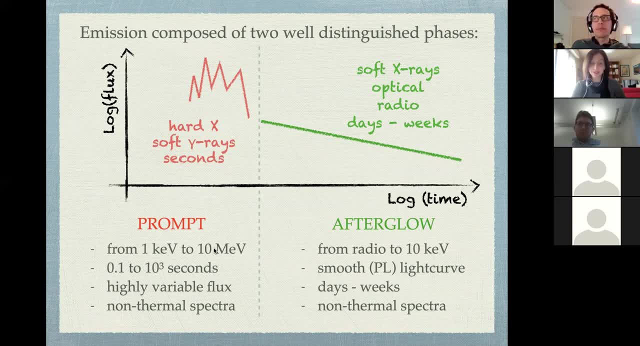 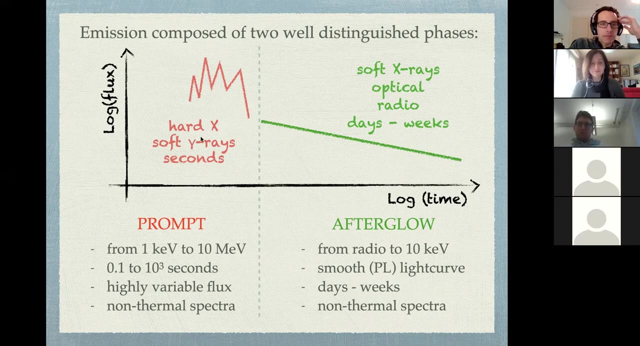 so we are talking about KeV, MeV, energy range. The duration of this emission ranges from fraction of seconds to, in the most extreme cases, thousand of seconds, And the flux is highly variable and spectra of the prompt emission are non-thermal. Then, immediately after the prompt, 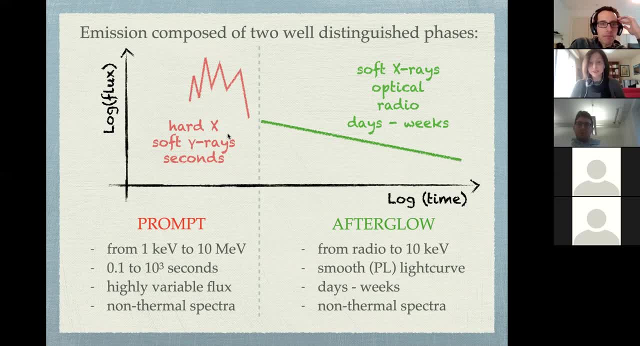 or sometimes it's even detected simultaneously to the prompt. we start detecting what is called the afterglow radiation, that is detected at longer wavelengths. So from soft X-ray we have optical and sometimes we also have radio detections. The flux decays in time as a power law. 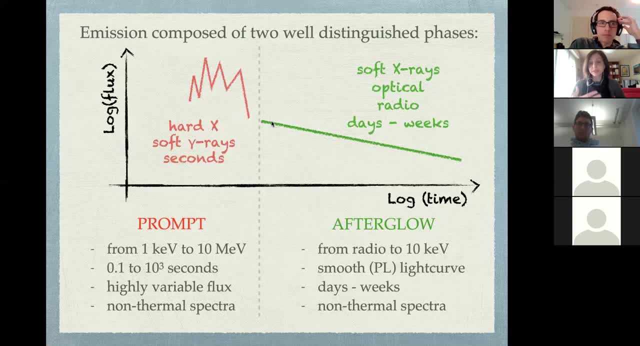 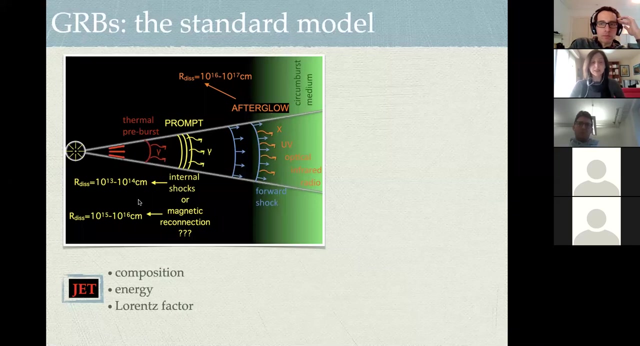 This emission is visible for several days, weeks or even months in the brightest cases, after the end of the prompt radiation, And also in this case the spectra are non-thermal. So this is a general a description of the standard model that we use to explain prompt and afterglow radiation. 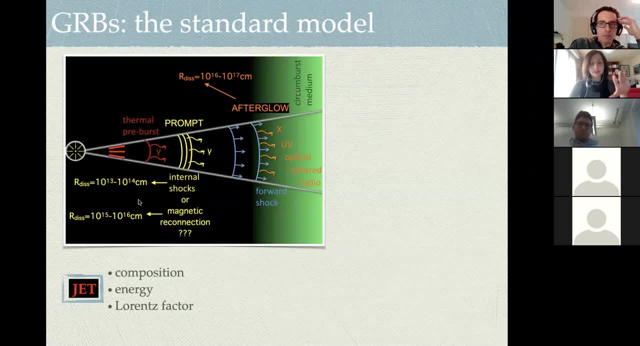 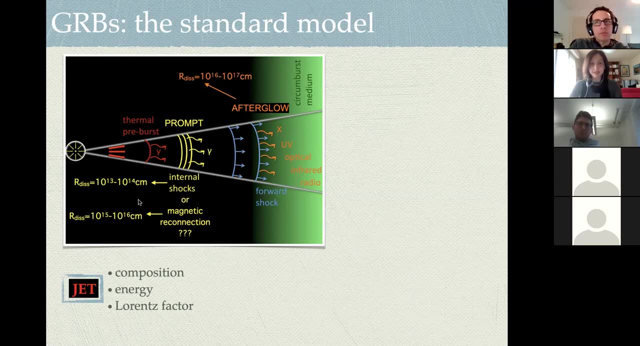 from gamma-reverse. So this is not an instantaneous picture of the gamma-reverse. It's more in evolution in time. Some gamma-reverse are transient sources, so we start from a central engine that is most likely a stellar mass black hole surrounded by an accretion disc. 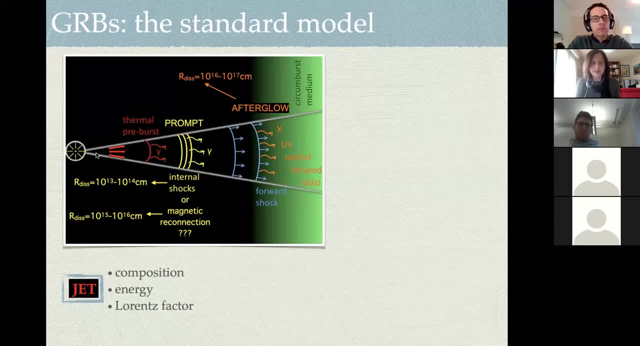 So, as the matter is created by the black hole, an outflow is launched. So we have an outflow of ultra-relativistic matter and radiation and magnetic field that travels with large factor, probably several hundred, And this outflow is collimated, probably. 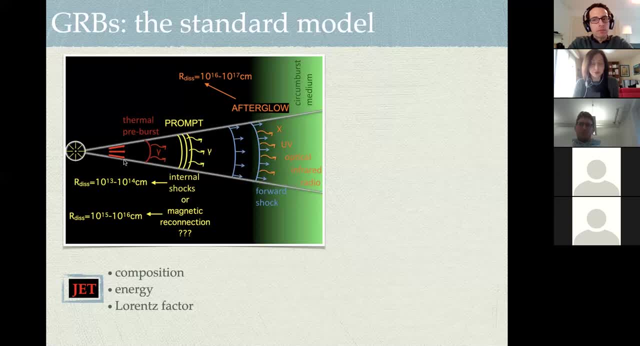 in two opposite jets, so it's not isotropic, And when this jet becomes optically thin, we expect to see radiation coming out from the jet in the form of a thermal component. What we see is non-thermal, so probably this radiation is a subdominant. 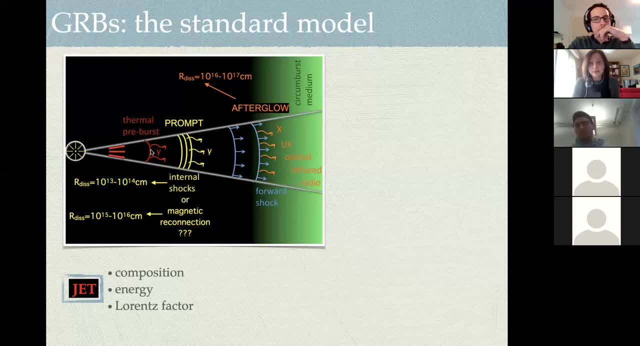 So most of the energy is either in the bulk motion of the particles or in the magnetic field. And here there is the first open question of gamma-reverse: What is the composition of the jet? What is carrying the energy? Is the magnetic field or are the particles? 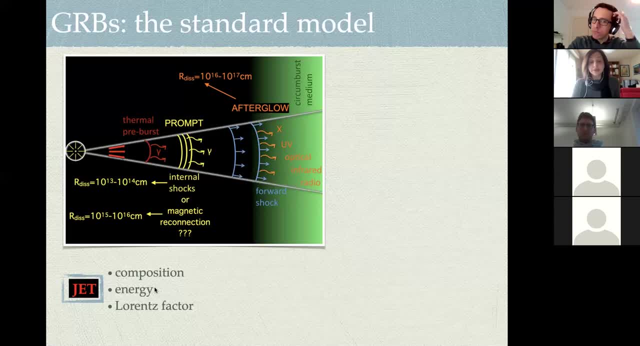 with the bulk motion. Second question is the energy carried by the jet. So what we see from gamma-reverse is electromagnetic radiation. So it's the part of the energy of the jet that has been converted to radiation, And we don't know this efficiency for conversion. 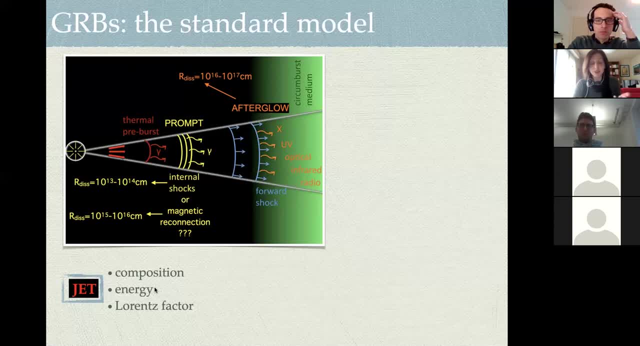 to electromagnetic energy. And then the other uncertainty is on the jet opening angle. So usually we estimate from the luminosity that we receive from the gamma-ray burst. we estimate the isotropic equivalent energy of the emission, which means assuming that the emission is 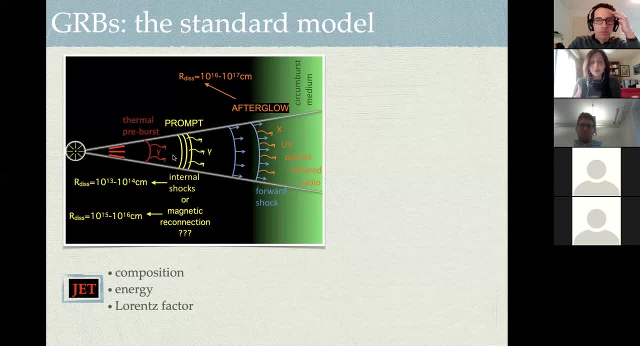 isotropic but most likely is collimated into two jets, And only if we can measure the jet opening angle we can derive the true energy of the emission and have a lower limit at least on the energy carried by the jet. Also, the Lorentz factor is difficult to measure. 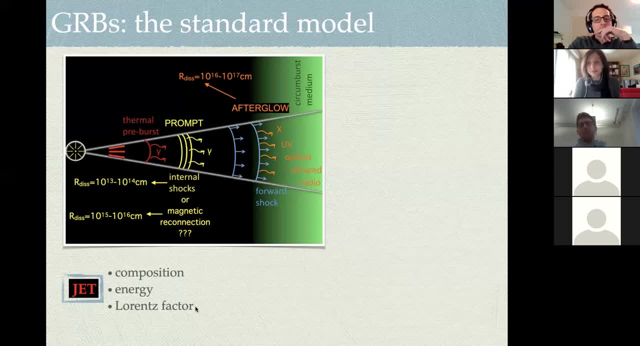 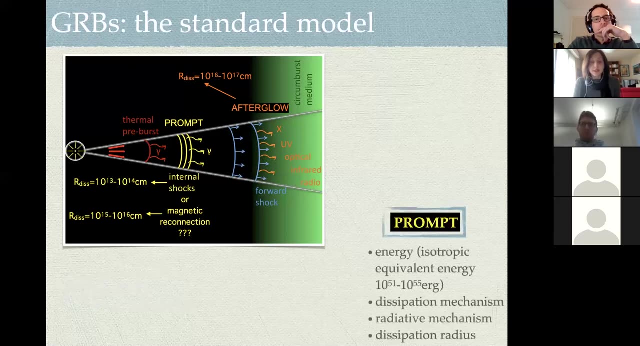 So we know, by several arguments or estimates when it's possible, that it must be of the order of 100. But the Lorentz factor distribution of gamma-ray burst is quite unknown. Then we see prompt emission, which means that the jet at some point must dissipate the energy. 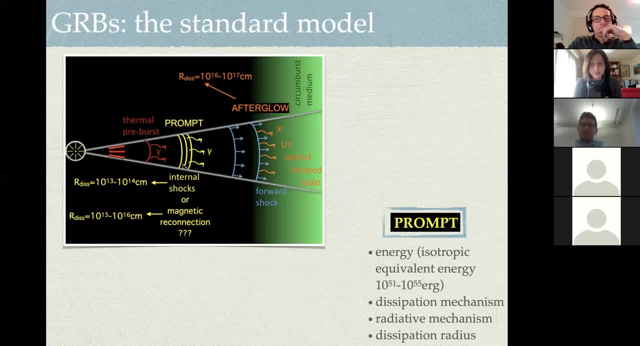 and accelerate particles, And then these particles will radiate a non-thermal spectrum, probably synchrotron radiation. So the dissipation mechanism, The nature of the dissipation mechanism, is uncertain because it depends on the nature of the jet. If the jet is matter-dominated, we 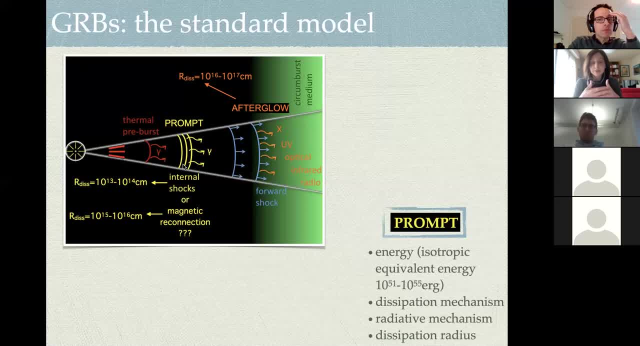 expect dissipation that can take place through internal shocks. So imagine that the outflow is not homogeneous, but is composed by different, well-separated shells. is an approximation, of course, And if the shells have slightly different velocities, they will dissipate the energy. 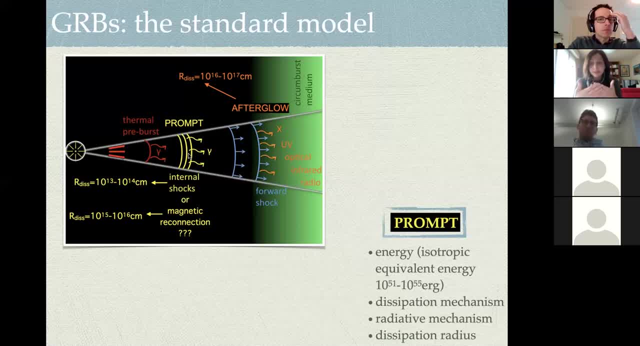 They will collide and produce these internal shocks that can accelerate particles, amplify the magnetic field and we expect to see synchrotron radiation. In the other scenario, if most of the energy is in the magnetic field, then we can dissipate part of the energy through magnetic reconnection. 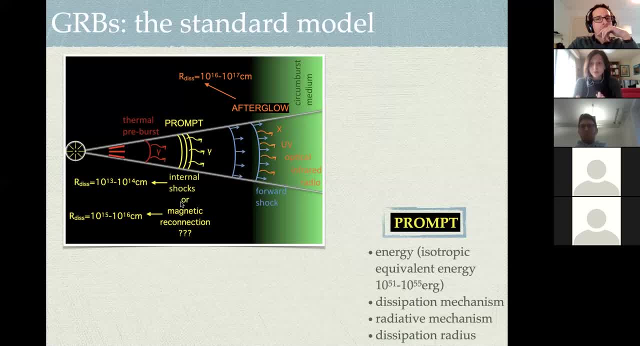 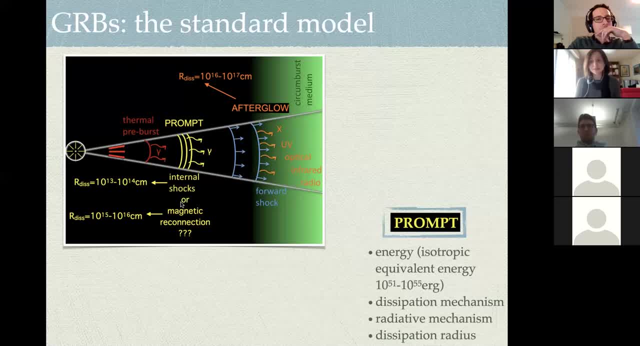 So the prompt emission is probably the least understood part of the gamma-ray burst physics. We don't know the nature of the dissipation mechanism. The synchrotron emission is not consistent with the spectra that we see, And we don't even know exactly where. 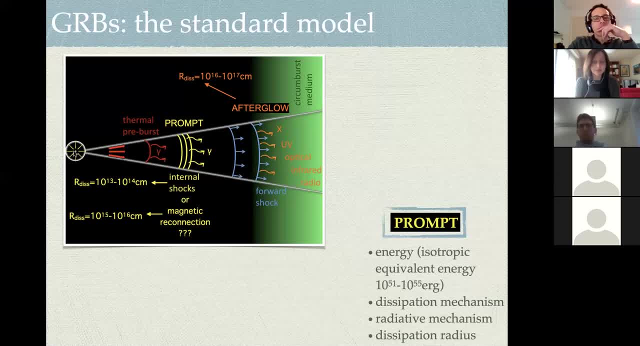 the dissipation takes place. So what is the dissipation? It's the distance between the emitting region and the central engine. So for internal shocks it's estimated to be around 10 to the 13, 14 centimeters, while for the magnetic jet it can be a bit larger. 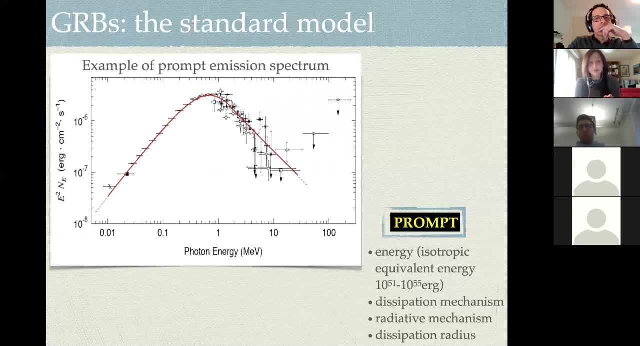 This is the typical spectrum from the prompt emission of gamma-ray bursts. So it's described by power loss at low and high energies And there is a peak where most of the energy is radiated. And if you compare this photon index with what you expect, 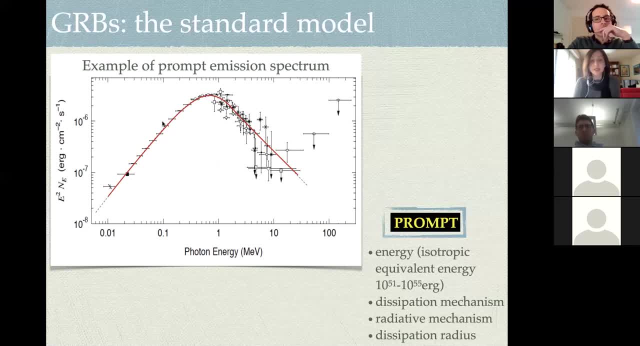 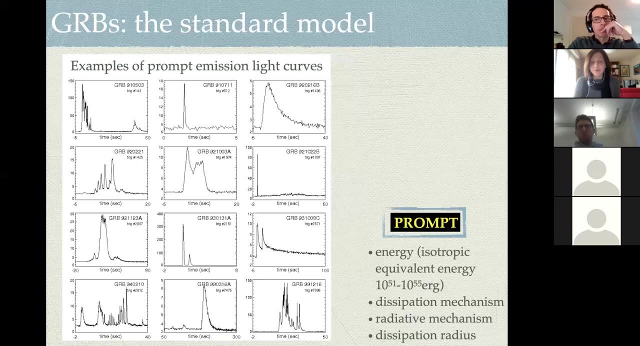 from synchrotron theory. there is an inconsistency, So we really don't know yet what is the mechanism, the radiative mechanism producing prompt emission in gamma-ray bursts. These are different examples of prompt light curves, So, as you can see, there is no typical light curve. 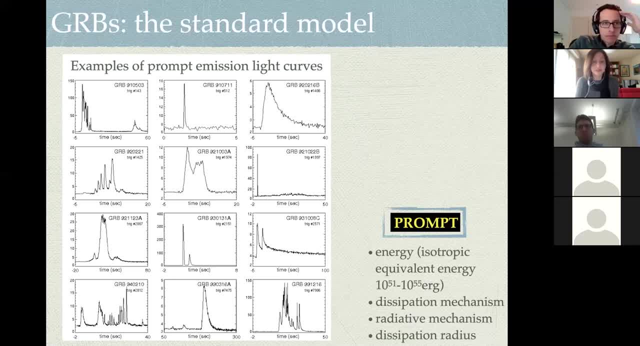 You can have different morphologies: one single peak, or more well-separated peaks, or very complex behavior. Now, if you take a large sample of gamma-ray bursts and start measuring the duration of the prompt emission, which is called T90, so T90 is a parameter that 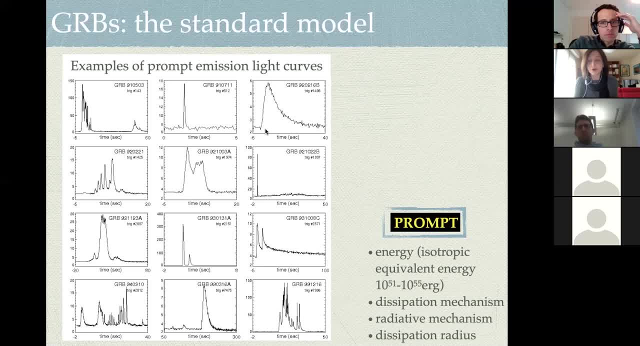 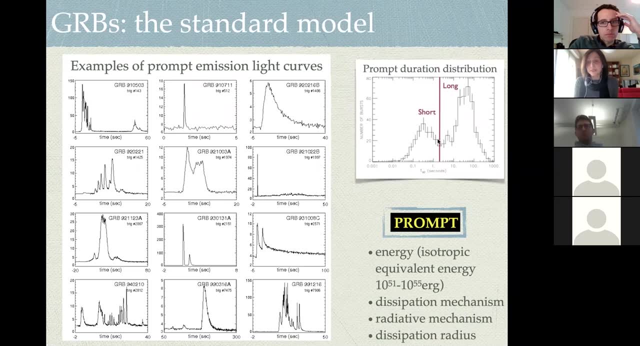 is used to estimate the duration of the prompt emission, you'll see that the distribution is by model. so this was the first hint for the existence of two different classes of gamma-ray bursts. short, if the prompt emission lasts less than two seconds. 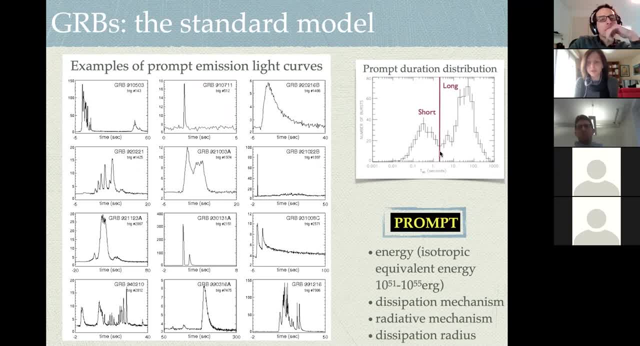 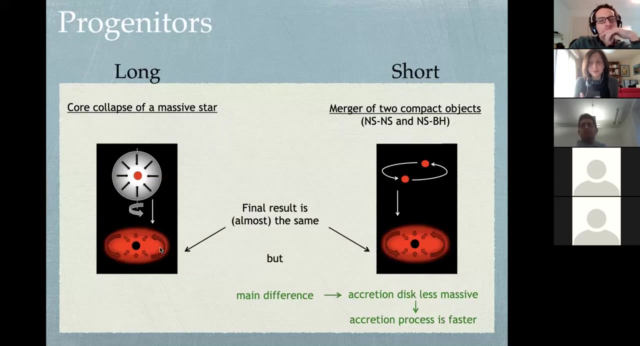 or long gamma-ray bursts. if the prompt emission lasts longer than two seconds, The difference is probably due to a different progenitor. So the final system- central engine that is in a creating black hole- can be produced through different channels. So for long gamma-ray bursts, we believe 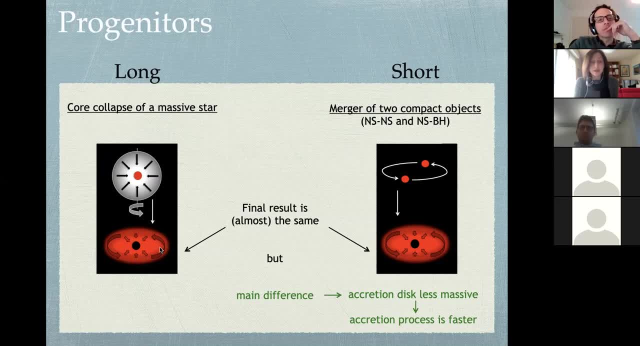 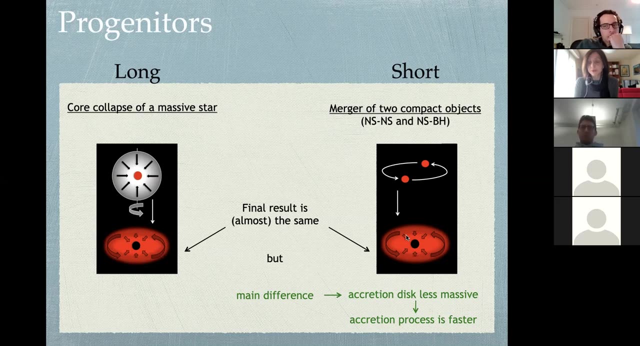 that the progenitor is a massive star and the core collapse of the massive star produces the black hole plus an accretion disk For short gamma-ray bursts. instead, we need to invoke the merger of two neutron stars, or a neutron star and the black hole. 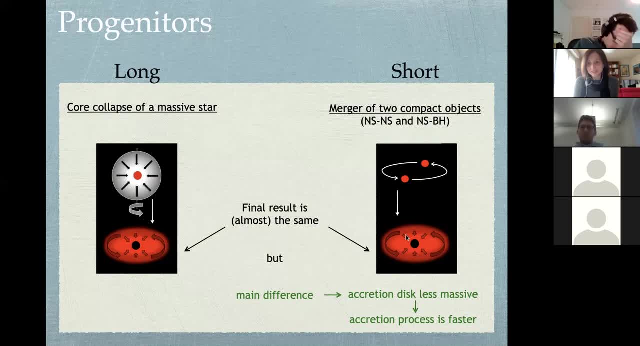 Since 2017, we have been working on a new method for short gamma-ray bursts and we know that neutron star- neutron star merger can indeed produce short gamma-ray bursts, because a short gamma-ray burst was detected in association with a gravitational wave signal from the merger. 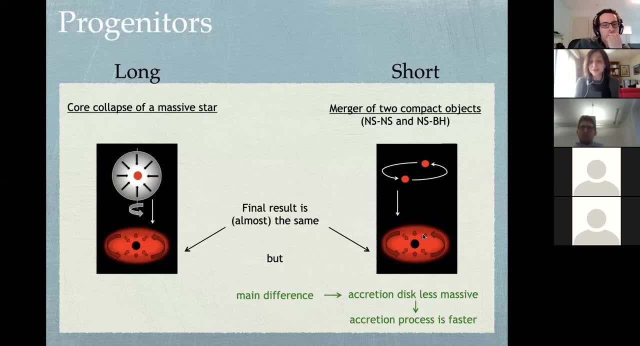 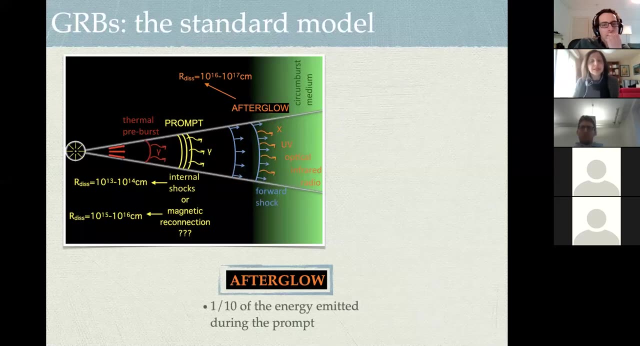 of two neutron stars And we still need confirmation for the possibility to produce short gamma-ray bursts in connection with a merger of neutron star and a black hole system. OK, So after the prompt We detect the afterglow radiation. So now you can imagine that the fireball 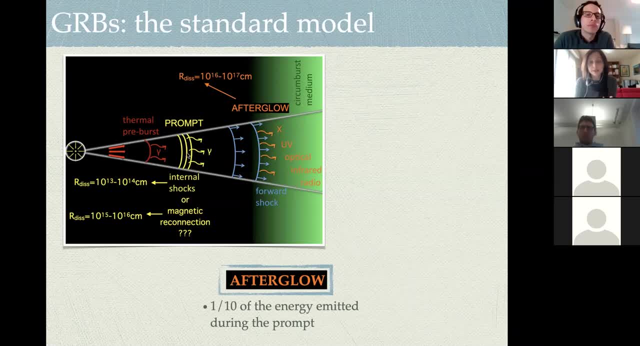 behaves like a homogeneous shell. So all the dis-homogeneities internal to the jet have been deleted. So in first approximation we can imagine a single shell that is expanding into the external medium, And at some point the external medium will start to affect. 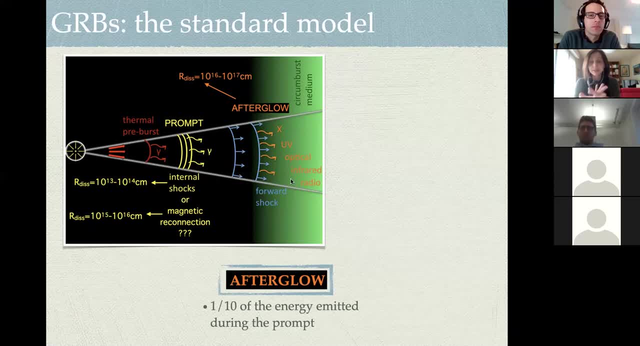 the dynamic of the jet. So the jet starts to decelerate, A shock wave travels into the external medium- the so-called forward shock or external shock- And the particles of the external medium are accelerated. The magnetic field is amplified And again we expect to see synchrotron radiation. 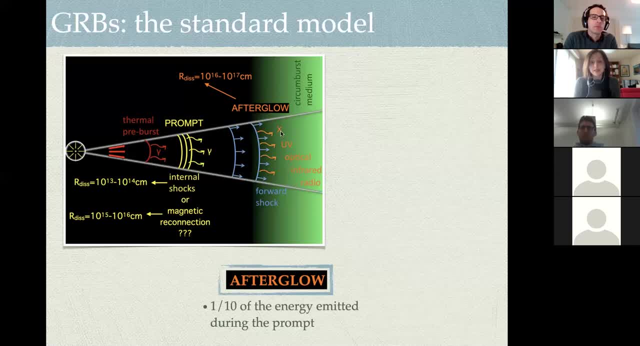 from the accelerated electrons, And this is the interpretation for what we see in X-ray, optical And radio band. So usually the radiation emitted in the afterglow is smaller, much smaller than what we see in the prompt. This means this implies that the prompt was very efficient. 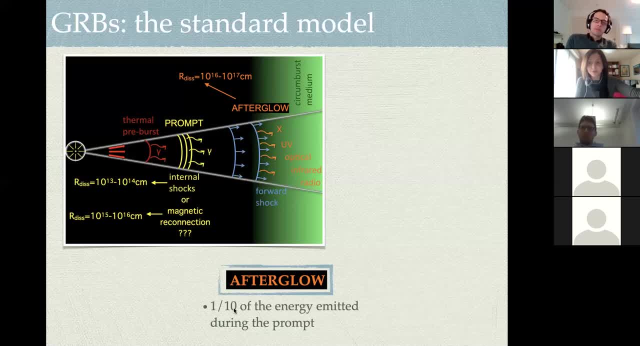 And only a small fraction of the energy is left for the afterglow radiation. This argument led to prefer magnetic reconnection over over internal shocks, Because internal shocks are a very inefficient way to dissipate the energy of the jet. And then, in case of internal shocks, 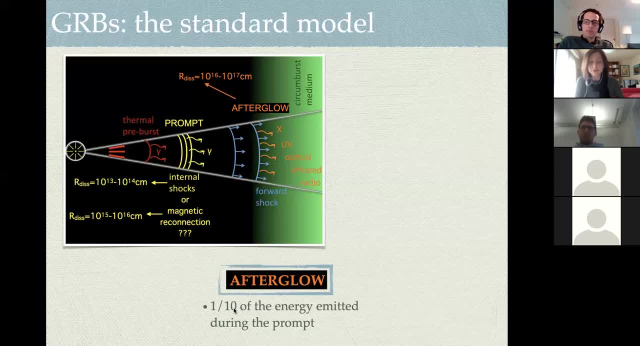 we would see a lot of energy available for the afterglow. So this was one of the main arguments- or maybe the main arguments- to start focusing on magnetic jets and magnetic reconnection and abandoning the general standard mode of the afterglow that instead invokes matter dominated jets. 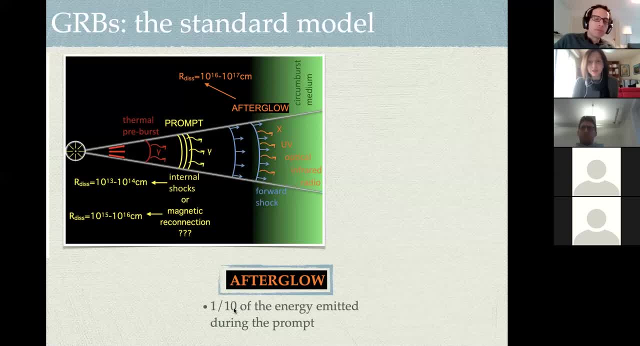 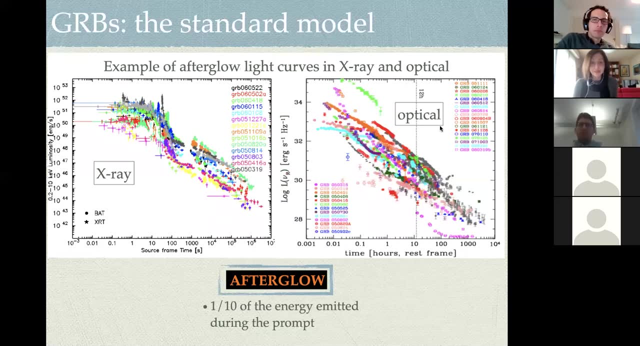 and internal shocks as dissipation mechanism. These are examples of afterglow light curves in X-ray here and optical in the other panel. So you see many different gamma reports. This part is still prompt radiation so detected by bat. So these are swift observations. 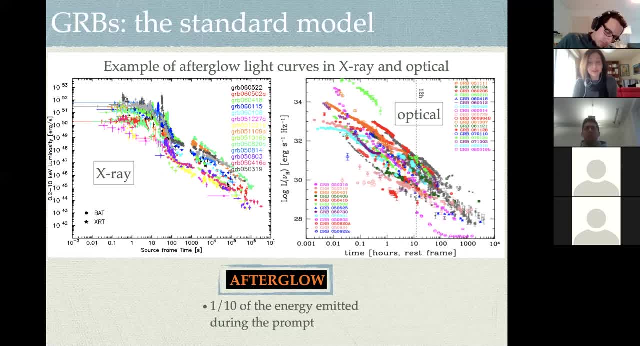 starts around here, so you can see that the flux decays in time as a power law. and actually these are all nice cases where the theory and the observation agrees quite well. but very often we see features in the X-ray that we cannot explain with a single model. 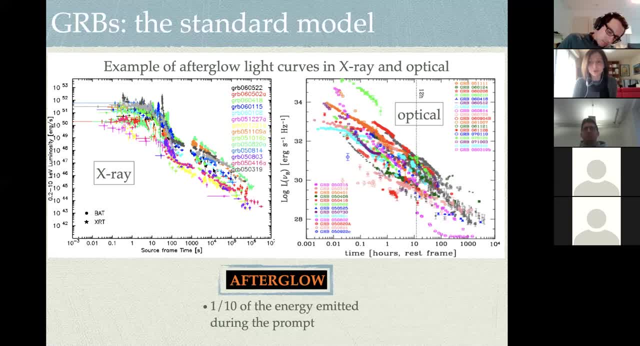 with a simple model, like flares or plateaus extending up to 10 to 4 seconds or re-brightenings. that cannot be explained with a simple model and we need to invoke more emission components, And here you see several examples of optical light curves. These in general behave as expected as single power laws. 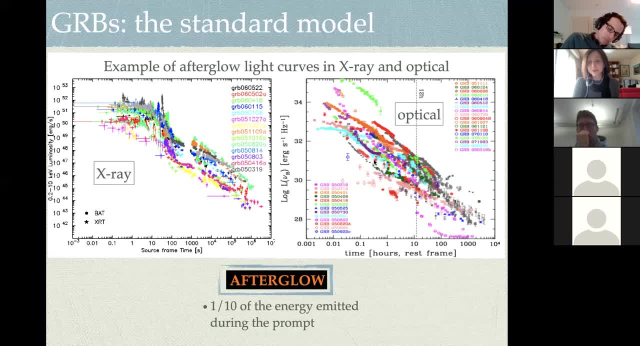 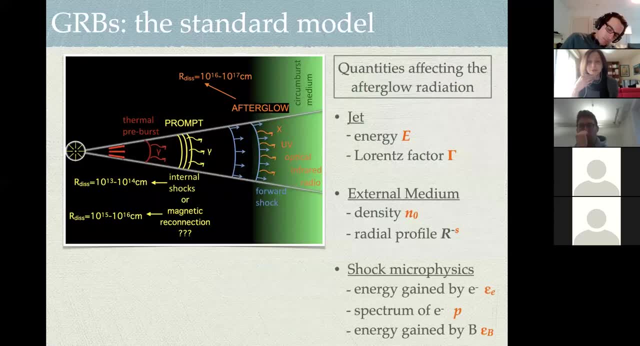 but also in optical sometimes we have features that are still not well explained. So the afterglow: it's in any case better understood that the prompt emission and, in principle, we would like to use afterglow observation to learn about the physics of gamma-ray bursts and of the environment because, as you can imagine, 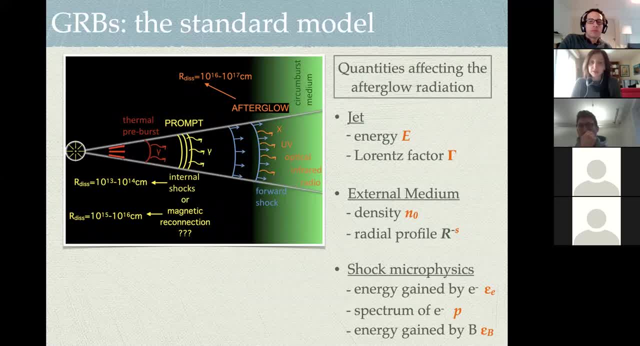 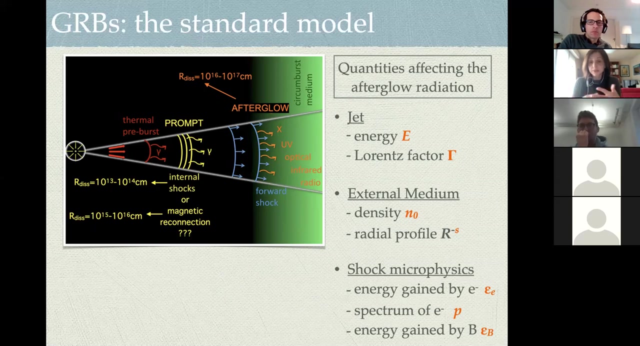 the final radiative output that we detect in afterglow and the afterglow phase is due to the interaction between the jet and the external medium. so it means that the radiation that we see is affected by the properties of the jet and in particular energy and Lorentz factor, and is affected by the properties of the circumvosed medium. so the density and the density profile. 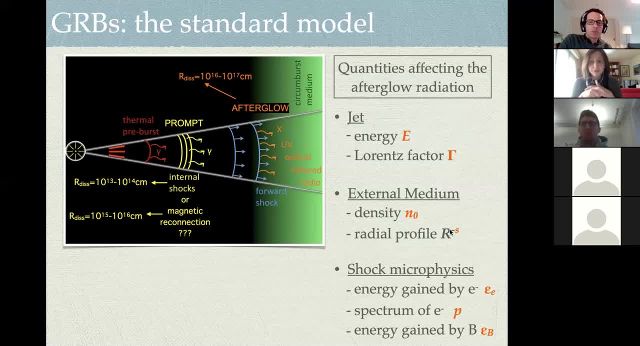 The radial profile of the external medium gives a lot of information about the progenitor. for long gamma-ray bursts we expect homogeneous medium with very low density. for long gamma-ray bursts we expect the medium shaped by the wind of the stellar progenitor. so we expect to learn also about the last phases of the stellar evolution. 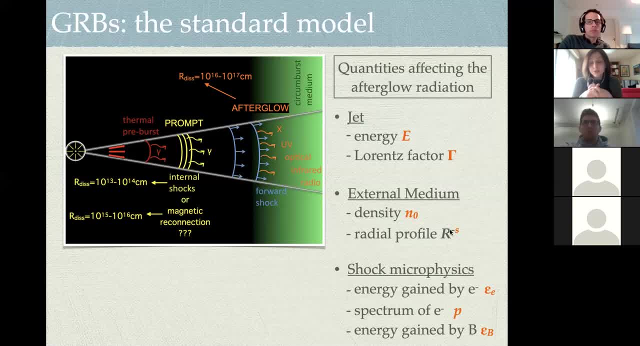 And then the afterglow radiation will also depend on the physics of the relativistic shocks, so in particular, will depend on the fraction of dissipated energy that is used to accelerate the electrons, will depend on the spectrum of the accelerated electrons and also on the fraction of dissipated energy that is used to amplify the magnetic field. 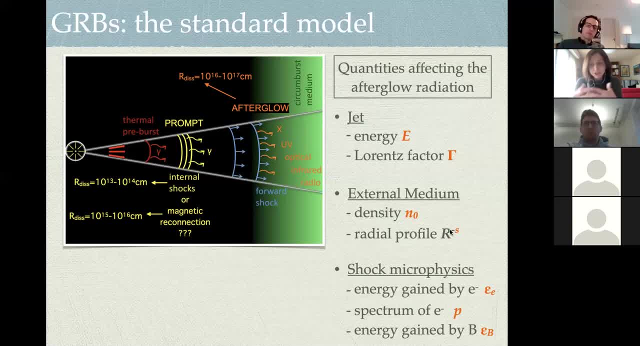 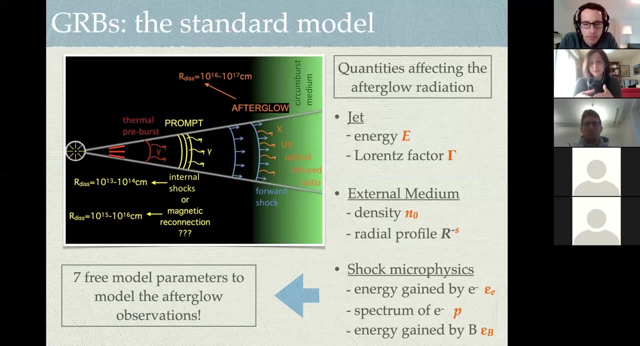 So, as you can see, the afterglow radiation, its shape and luminosity, depends on seven parameters. so very often it's difficult to use afterglow observation to constrain all these parameters. also because in general, in average gamma-ray bursts we don't have well sampled light curves at all wavelengths. 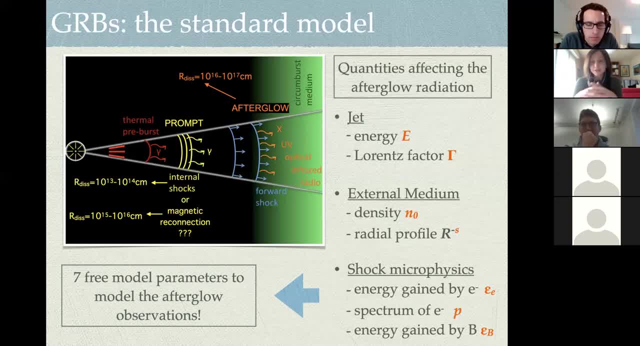 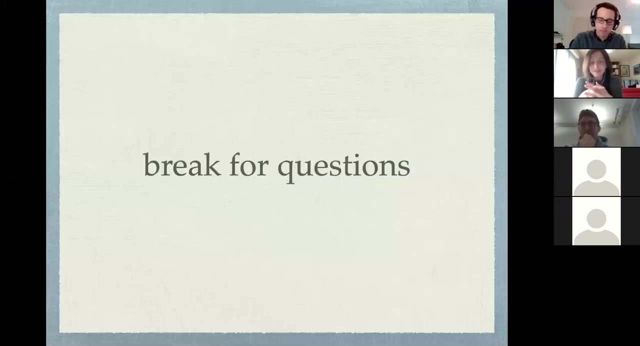 So, unfortunately, the potential of afterglow radiation to learn about all these physics from the external medium to progenitors, the jet, the relativistic shocks, is very limited by the fact that there are strong degeneracies among all the three parameters. Okay, so after this general brief introduction on gamma-ray bursts, that will be necessary to understand the second part. 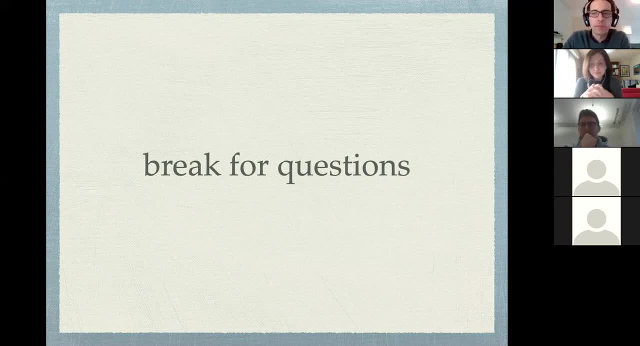 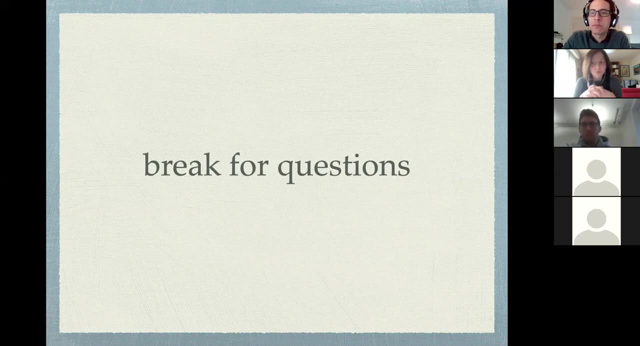 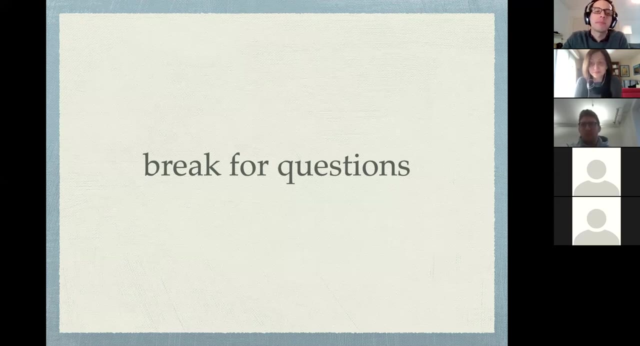 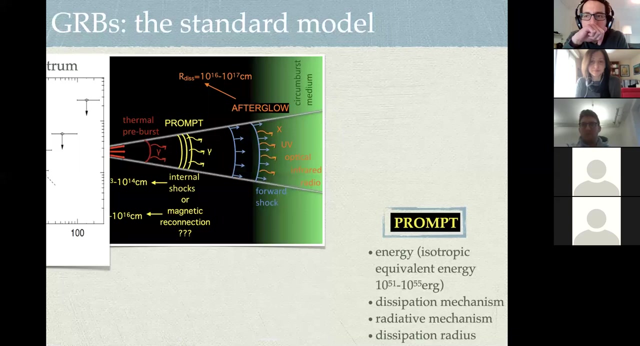 I would like to stop and see if you have questions. We have one actually. okay, may I Sure? So thank you. So in the slide where you're showing the typical spectrum of the prompt emission. so this is like an integrating, an integrated spectrum, I guess here. perfect. 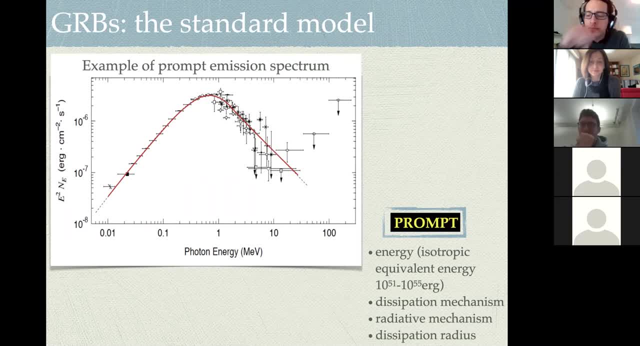 Yeah, and so, yeah, I was wondering, like: so you were saying that the slope, the typical slope you would expect from synchrotron emission is not the one that you see on the data, and like, what is actually your expectation and why it is inconsistent with the data. 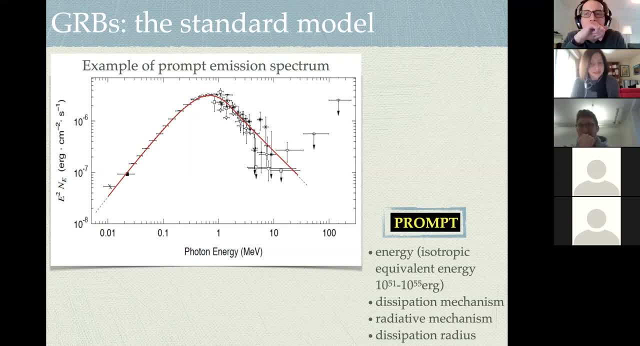 This was my question. Yeah, sure. So the main inconsistency is that very often we see spectra that are harder than the synchrotron spectrum. So the synchrotron spectrum depends also on the injection spectrum of electron. I guess This high energy part yes. 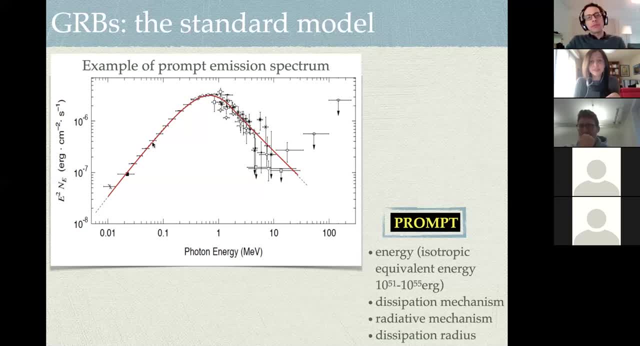 This depends on the spectrum, But this is dominated by cooling. This is only defined by cooling because this is a delta injection in time. So this is not a steady state equation that you solve, I guess. Yes, exactly, You have injection, continuous injection, for limited time. 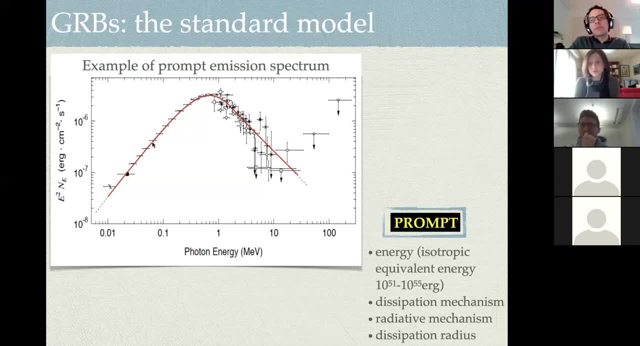 And so you can follow: this is fast cooling, So particles, in any case, cool Very rapidly And what you see here is the cooling part of the emission. Okay, Okay, Very good, I understand, then. So, okay, And this is a part that is not consistent with expectation. 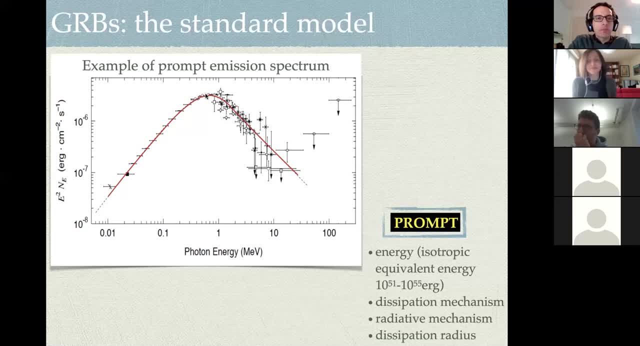 Yes, Yes, Because you have a clear prediction for the synchrotron. So you have a one third below the cooling frequency and then you expect something like minus 1.5 in photon index. So minus 0.5.. And you see, actually something that is in between these two values as average typical value of this photon index. 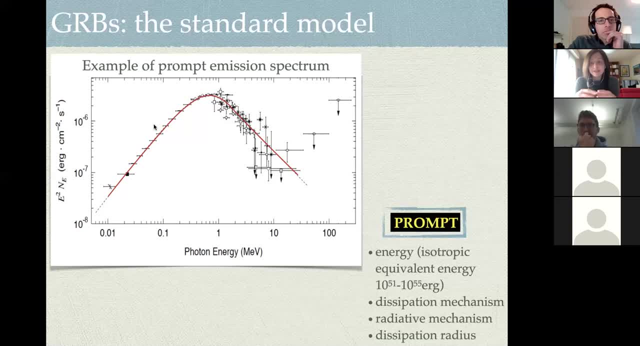 But in many cases you see something that is harder than one third, So it's really hard to explain which synchrotron model. Okay, Thank you very much. Okay, Tom has a question? I think, Yeah, Just one. 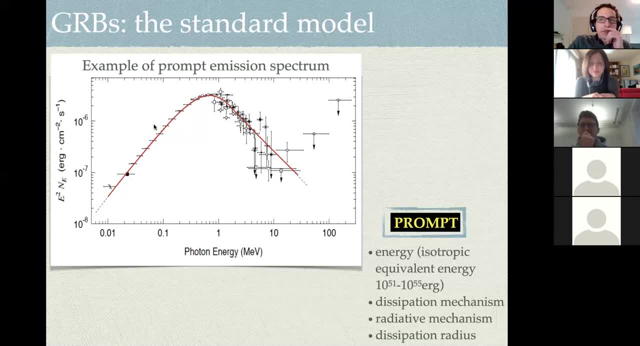 That's okay. I was wondering: is it known or are there theories about what makes the burst happen in the first place? So you have this object that's accreting for, I guess, presumably a very long period of time. What makes it suddenly burst, this big release? 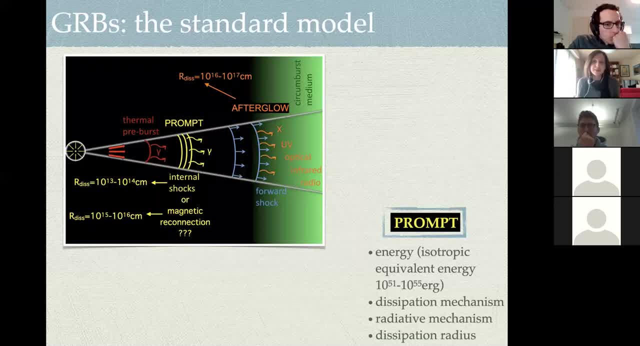 Oh no, no, The accretion is very short, because you have. so these are explosive phenomena. So when the compact object forms, it's so rapid, It's surrounded by this small accretion disk And as soon as it accretes the matter, it launches a jet. 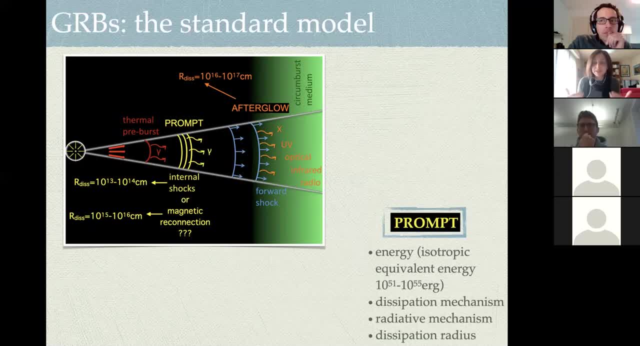 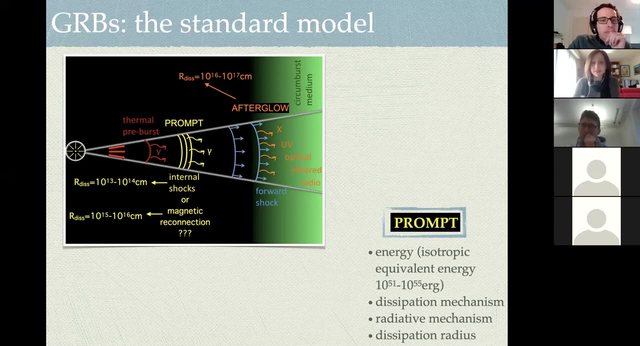 And that's it. And then the jet is not a steady outflow, So it's something. the outflow, the emission of this matter, lasts for seconds, And then we see an emission that has a similar time scales. I see, Okay. 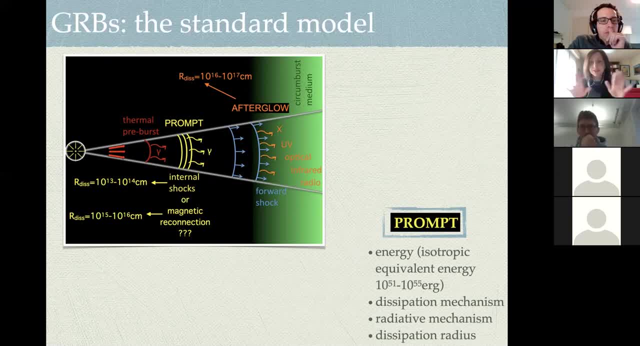 So it grabs a small amount or a large amount of matter, Yeah, And then the accretion stops. Once you accreted this matter that remained after the collapse or the merger, everything stops. So you just have this jet, this outflow that is traveling in the external medium and first produces, by internal dissipation, the front emission and then the afterglow radiation. 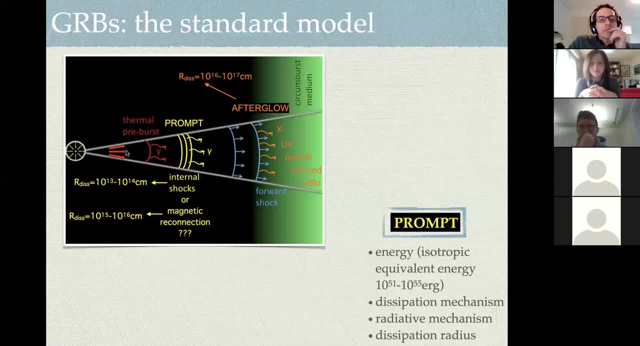 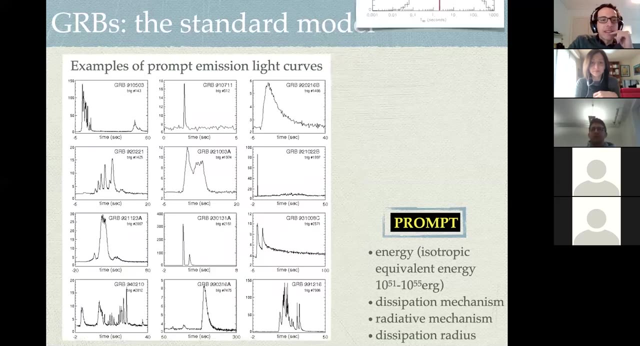 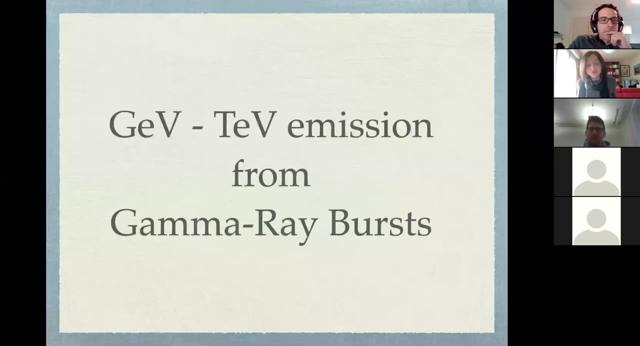 I see, Thank you. So the matter is basically the remnants of what was left when we formed the black hole in the first place. Yeah, I see, Thank you. I see no other questions, So please, Lara, go ahead. Okay. 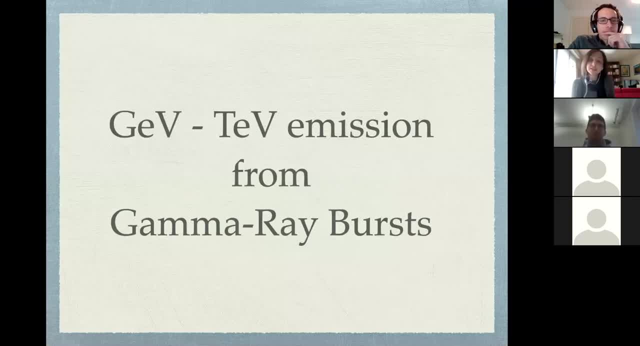 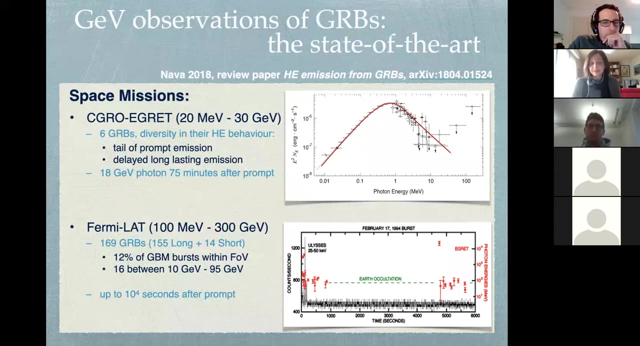 So in the second part I will focus on GV and TV emission from gamma-ray burst. These two energy ranges are studied with different instruments, So let's start with the GV radiation. We already knew with YGRET that gamma-ray burst emit also GV radiation. 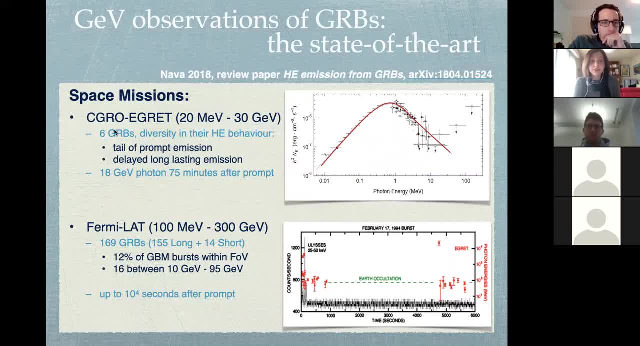 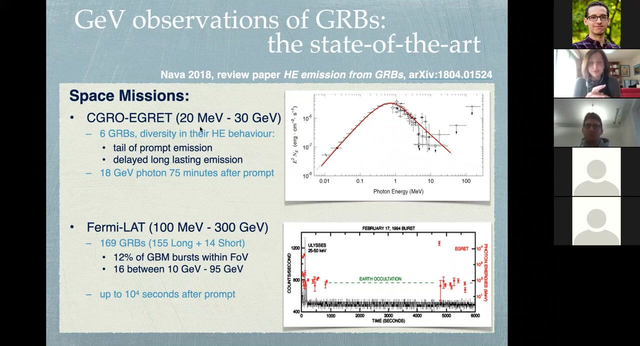 So YGRET was on board, the Compton Gamma-ray Observatory and the low energy instrument, so KVMEV instrument, But it detected almost 3,000 gamma-ray bursts And YGRET, at higher energies, detected only six of them. And so we are in this energy range 20 MeV to 30 GeV. 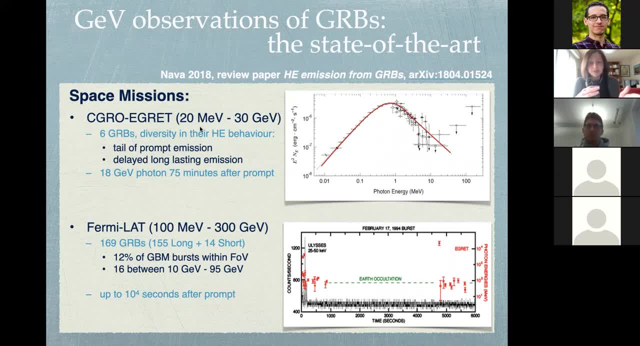 And even though the numbers are very small, it was already clear with YGRET that we are looking at different components. So GV emission can be sometimes just the tail of the prompt emission. So here again there is the prompt spectrum. So sometimes what was detected at 100 MeV or 200 MeV was consistent with being just the tail of what we see in the prompt. 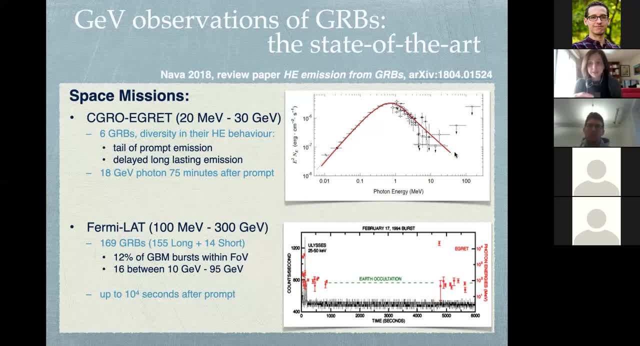 But sometimes YGRET clearly detected GV radiation at much later times, So when the prompt is already ended and during the afterglow emission. So probably already YGRET made clear that there is GV emission Or 100 MeV emission produced during the prompt. 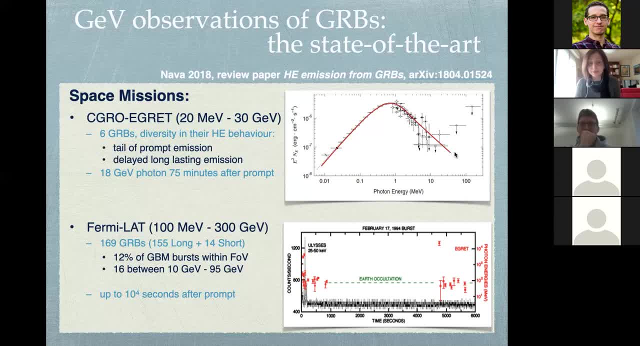 And there is also GV emission producing during the afterglow- Very famous this case here. So what we see in black is the prompt emission. So there is a spike here within 100 seconds and just background radiation And YGRET in red detected photons, both during the prompt. 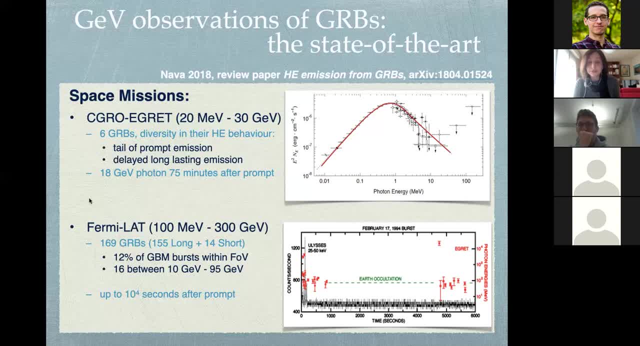 But also 18 GV photons 75 minutes after the prompt, So clearly related with the afterglow component. Now we detect gamma rebirth at GV energies thanks to Fermi-LAT, So these numbers are taken from the second LAT catalog of gamma rebirth that stops at 2018.. 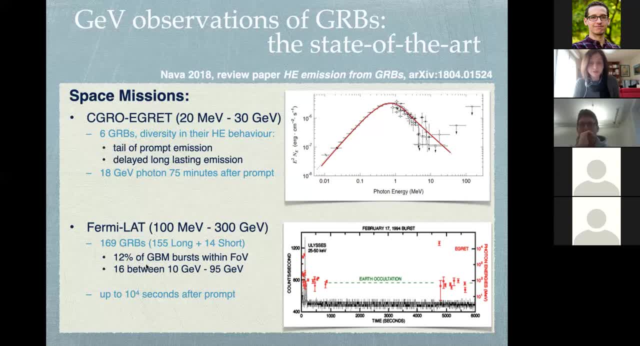 So 10 years of LAT observations of gamma rebirth And in total LAT detected 169 gamma rebirths, both long and short. This is a small fraction of the gamma rebirths detected in their prompt emission by the Fermi GBM. 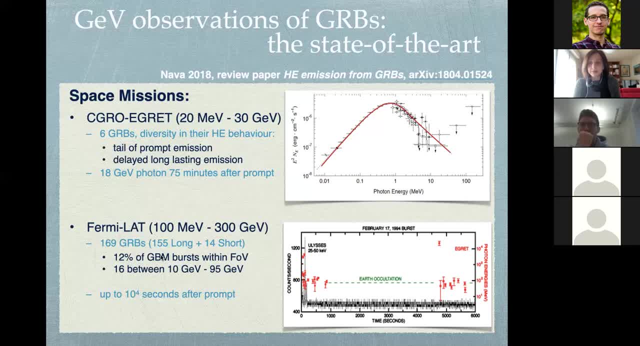 So GBM is sensitive in the KeV-MeV range, So detects prompt emission from many gamma rebirths- Four or five every week And only a few And only a small fraction of them is also detected at higher energies, And usually this emission is detected below 1 GV or around 1 GV. 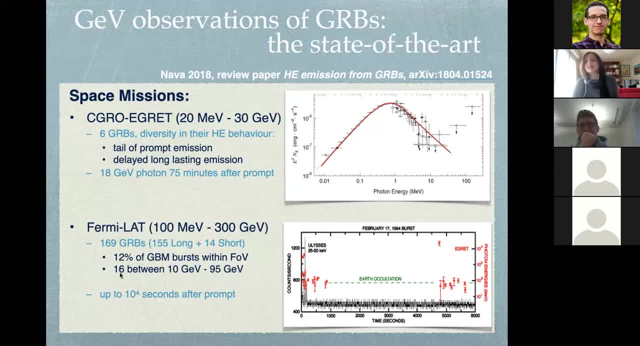 But in 16 cases there are photons detected above 10 GV And the record holder is this photon detected at 95 GV from a very bright gamma rebirth. LAT also discovered that this emission can last up to 10 to 4 seconds. 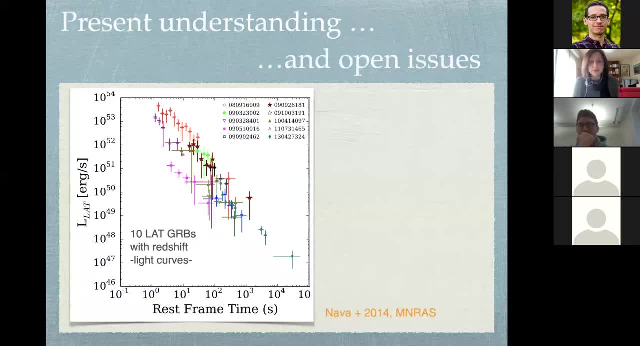 And so very long component. These are 10 examples of light curves of emission detected by LATs in the 0.1 to 10 GV range. So, as you can see, the flux decays in time as a power law. These are all gamma rebirths. we know redshift. 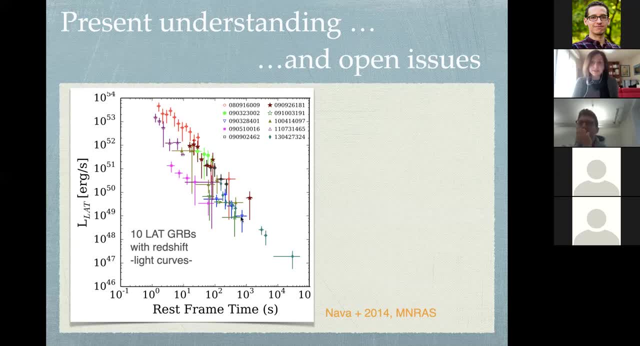 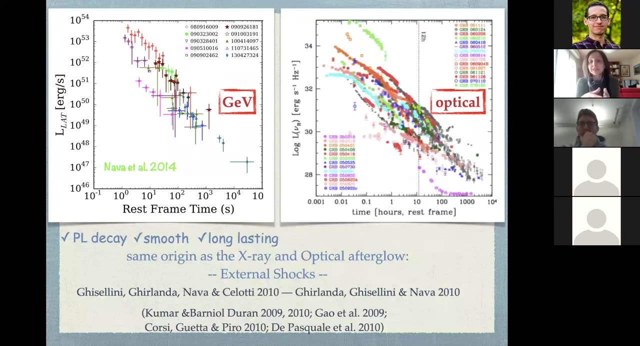 We used them in 2014 to study the origin of this emission and see if this is consistent with synchrotron radiation in the afterglow. So it's the high energy part of the afterglow spectrum. The similarity with the optical light curve is obvious. 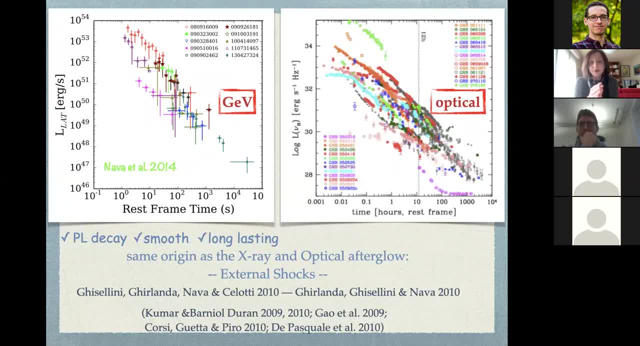 So you can see from this comparison that the behavior of this light curve is similar to what we see in the afterglow, For example in the optical. So there is no variability. It's a power law decay. It's very smooth and long lasting. 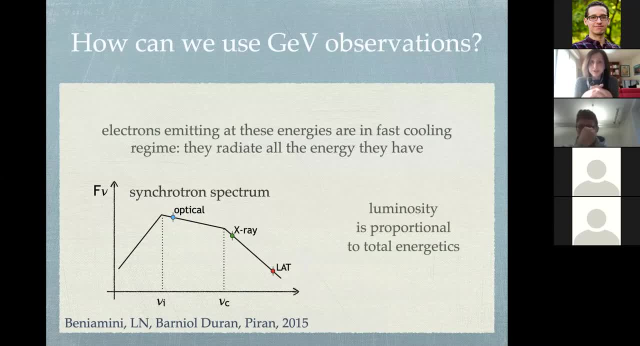 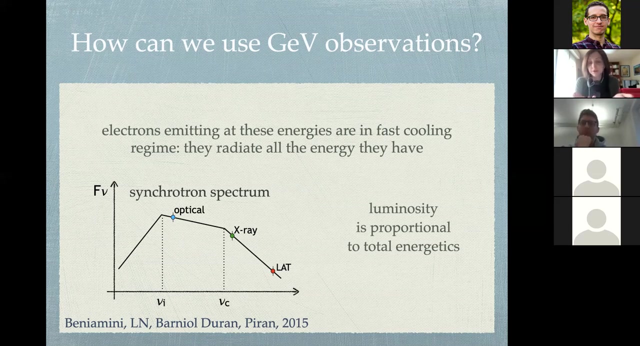 So if these observations of GV Radiation- in those cases where the emission lasts much longer than the prompt, So it's clearly associated to the external shock, to the afterglow radiation, How can we use them? If this is interpretation, how can we use them to learn about the physics of external shocks? 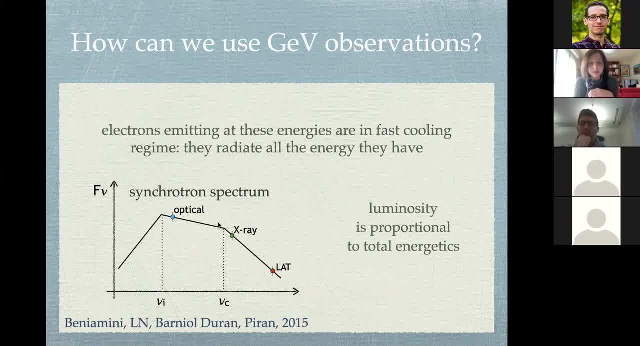 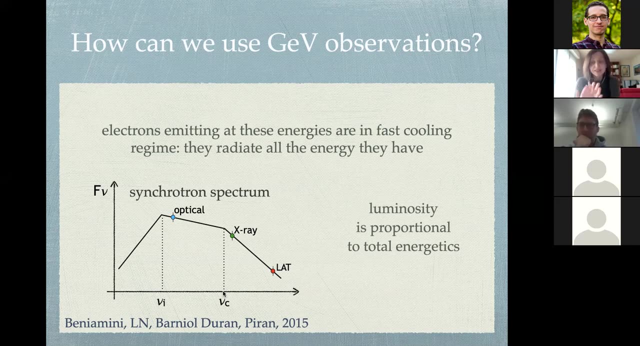 Well, there is something nice in observing the synchrotron spectrum as such a large energies, Because if this is the synchrotron spectrum, So here you have the cooling frequency. The afterglow is, for most of the time, except the very beginning, is in slow cooling. 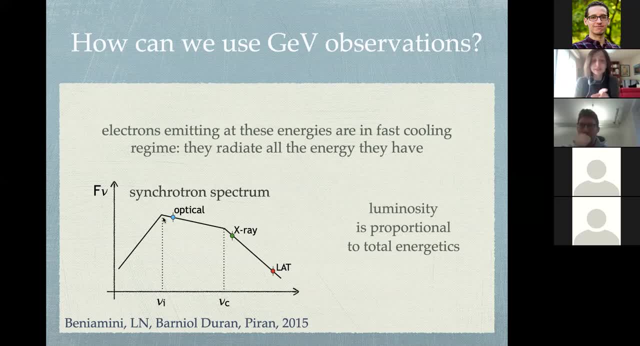 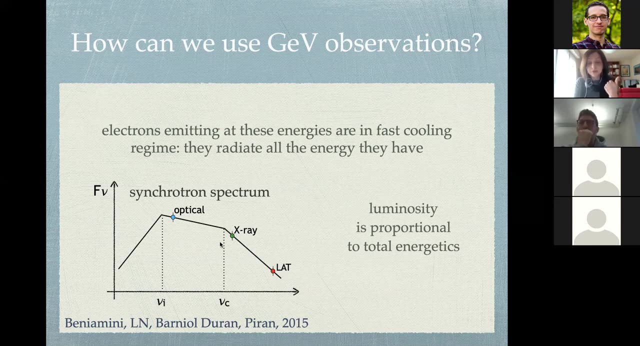 So here you have the cooling frequency. This is the synchrotron frequency corresponding to electrons with the minimum energy, And so you have two breaks in the spectrum, And this radiation here Above the cooling frequency, is produced by electrons that are in fast cooling. 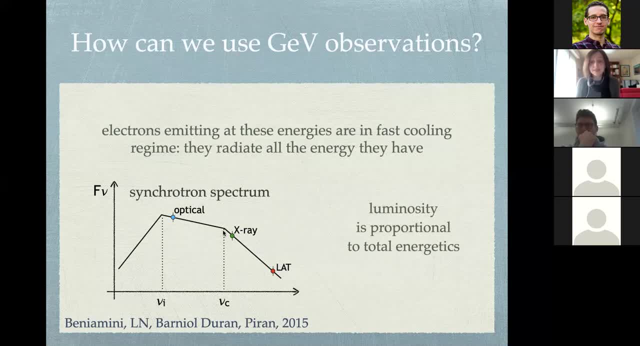 So they are emitting all the energy they have, no matter the magnetic field, no matter the density. So the flux here is quite independent from all the seven free parameters that we saw that we need to describe the afterglow. Here the luminosity just depends on the energy of the electrons. 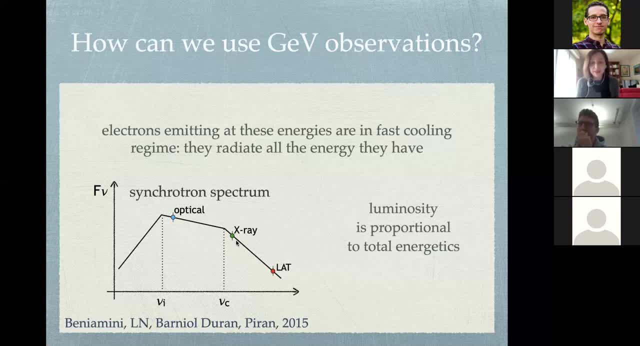 Because they will radiate all their energy. So this has been used with X-ray observation in order to infer a robust estimate of the energy of the jet. And this is quite important because if we know the energy of the jet during the afterglow emission, 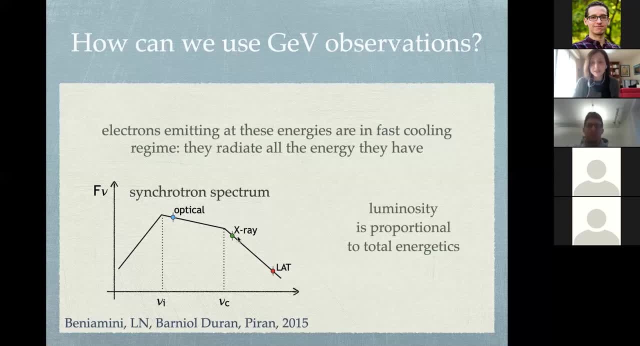 and we know the amount of energy emitted during the prompt radiation, we can estimate the efficiency of the prompt radiation. If the mechanism producing the prompt is very efficient, we expect to see a small amount of energy during the afterglow. Otherwise, if we see a lot of energy during the afterglow, 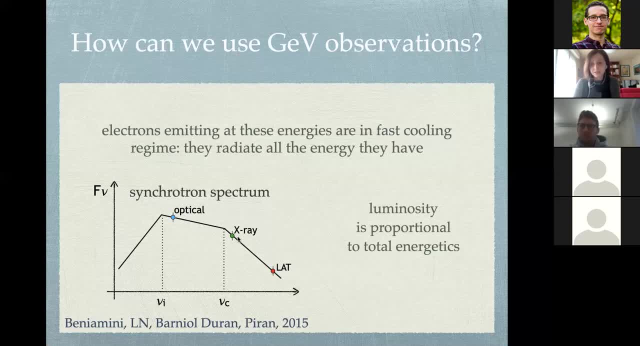 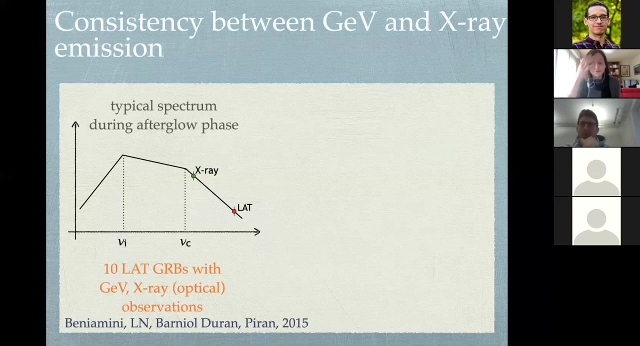 we can say that the emission mechanism producing the prompt was very inefficient, And then we can start deciding which model for the prompt emission and for the dissipation and for the jet composition is the better one. OK, so now that we have also GEV observations, 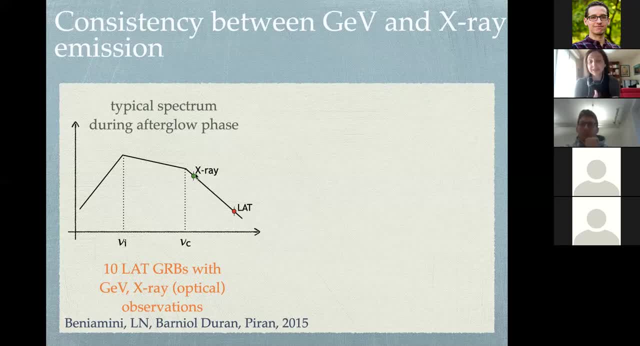 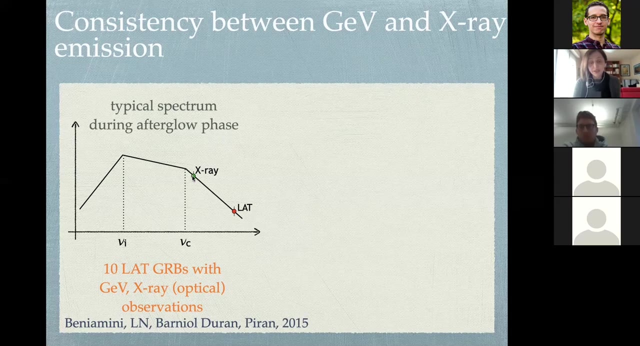 we can do the same exercise, Of course, if X-rays are above the cooling frequency. this is even more true for the GEV energy range. So in this case we took 10 gamma rebirths, First with LUT and XRT observations. 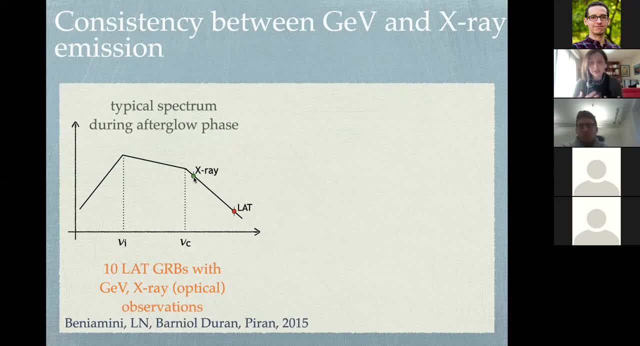 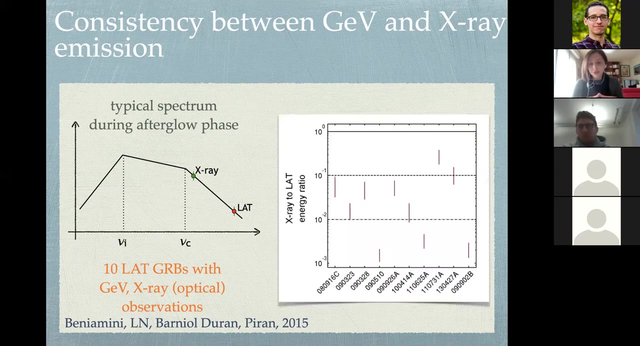 and estimate the energy of the jet starting from X-ray and LUT observation independently. Of course we need to infer the same estimate of the jet energy, But this is not the case. So the ratio between the energetic estimated using X-rays and using GEV radiation. 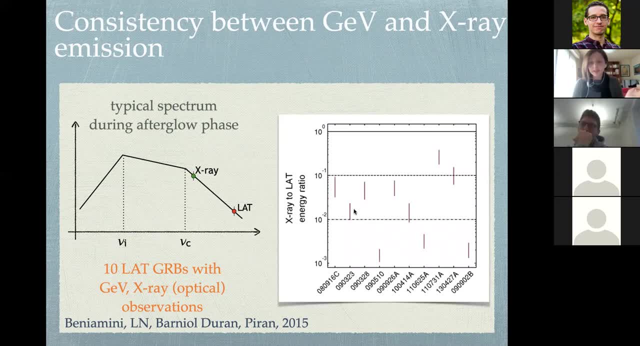 it's far from being one. So it means that the two different observations gives quite different results on the inferred energy of the jet. So it seems like the X-ray is less luminous than what predicted by the model, or the LUT is more luminous than what it should be. 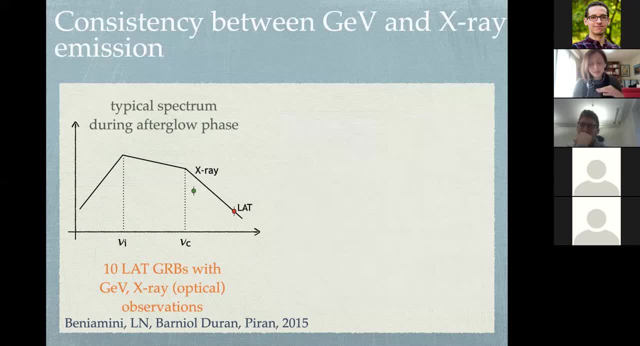 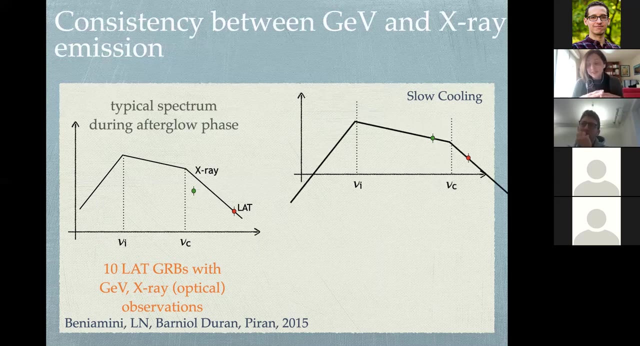 So by modeling these gamma rebirths, so performing a full modeling also with optical observations, we saw that the problem can be solved in two different ways. It also depends from the gamma rebirths. Sometimes, simply, the X-ray is below the cooling frequency. 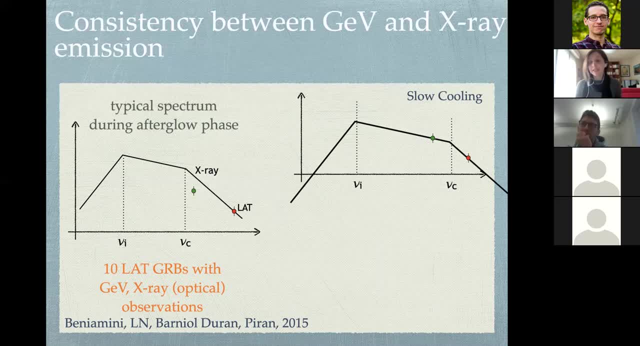 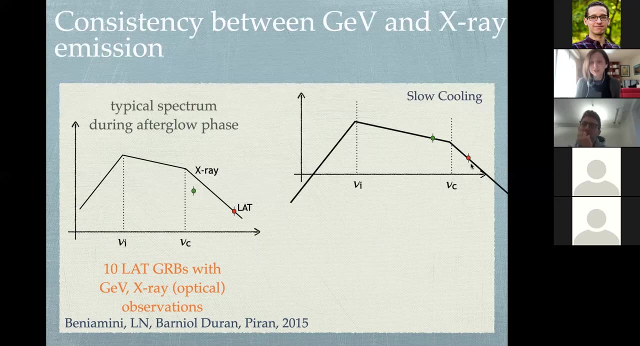 So the X-ray is not a good proxy for the energy of the jet, because it's emitted by electrons that are in slow cooling Instead, if the GEV range is above the cooling frequency. so the GEV emission is a good proxy for the energy of the blast wave. 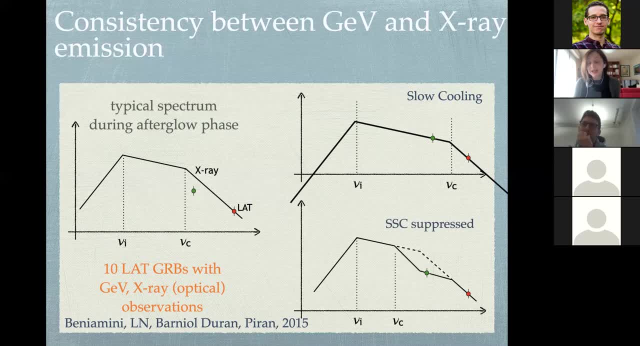 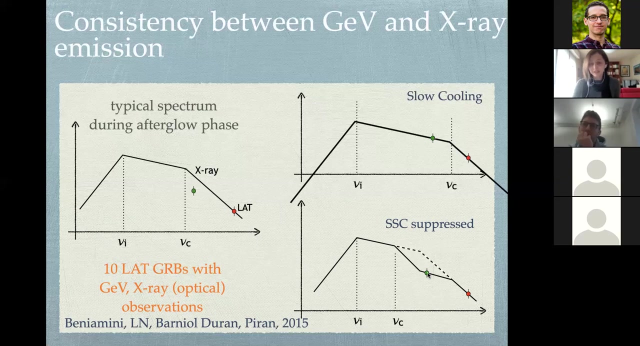 Another possibility is that the flux in the X-ray range is suppressed by inverse Compton cooling, So this part of the synchrotron spectrum is efficiently upscattered to another component at higher energies- an inverse Compton component, And the X-ray flux is then reduced. 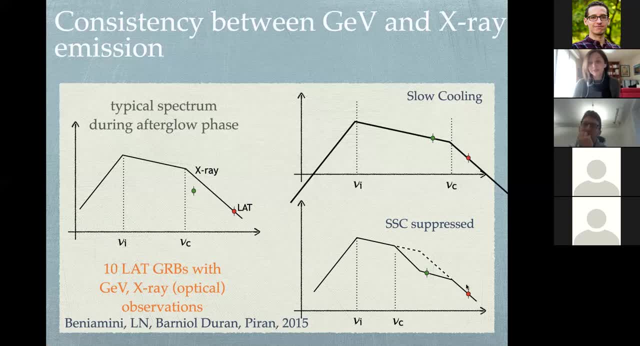 And this is not true for GEV energies, because at this point Klein-Nishina plays an important role. So this scattering occurs in Klein-Nishina regime, so the cross-section is very reduced and they are not efficiently upscattered to high energy. 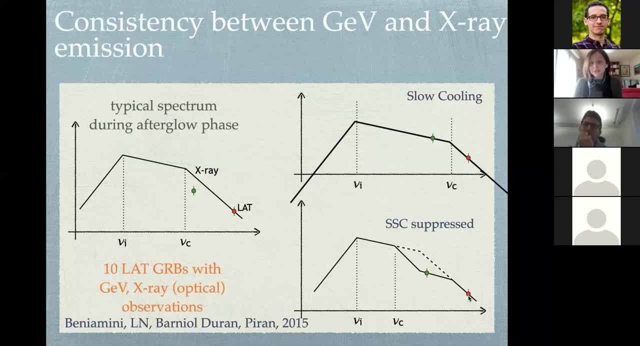 In both cases we see that the GEV emission is a more robust proxy for the energy of the jet And then it's a more robust proxy for deriving the efficiency of the prompt emission. And if we use this relatively new GEV observation from Fermi, 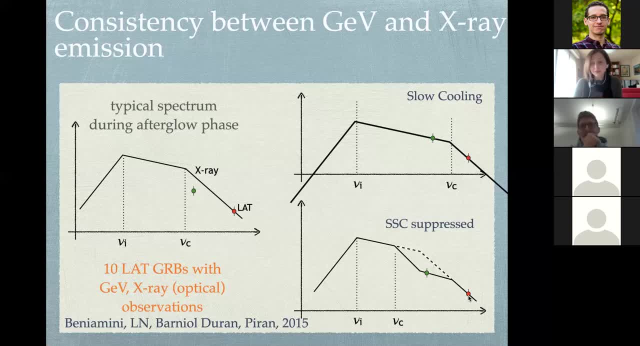 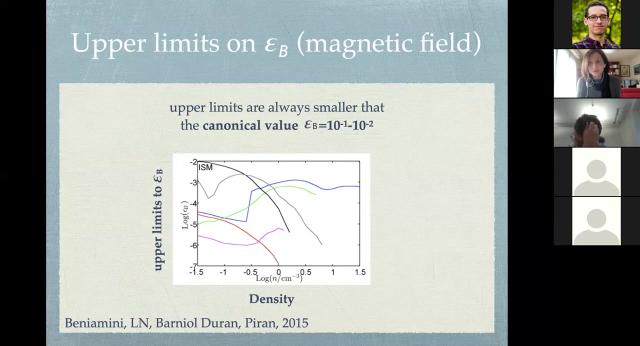 we can infer that the mechanism producing prompt emission can be an inefficient mechanism. Internal shocks are still a viable model to dissipate the jet energy and produce synchrotron radiation from the prompt emission. Another result of this modeling, using also GEV radiation, is that we could put upper limits on epsilon b. 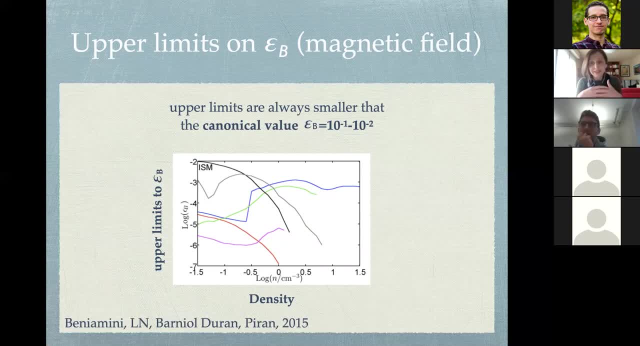 which is the fraction of energy dissipated energy by the external shock that is used to amplify the magnetic field. We don't know much about acceleration and magnetic field amplification at the external shocks. that are ultra-relativistic shocks And usually people assume. 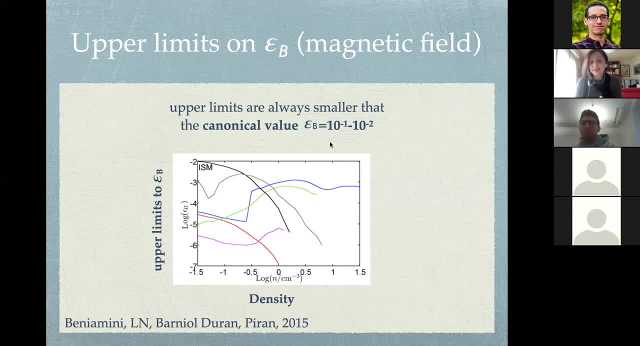 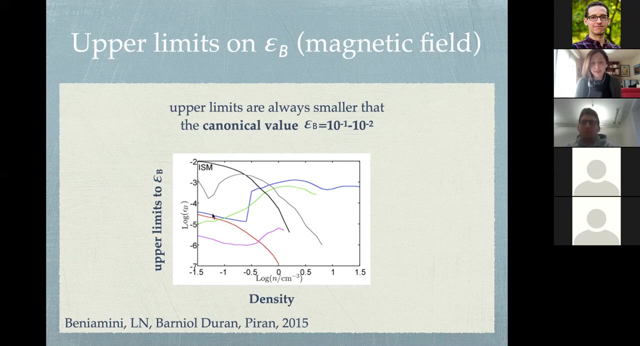 that this fraction that goes into the magnetic field is 10% or 1%, And here we demonstrated that actually the value of epsilon b must be much smaller to explain GEV observations, together with X-ray and optical. So this multi-wavelength modeling requires very small values of epsilon b. 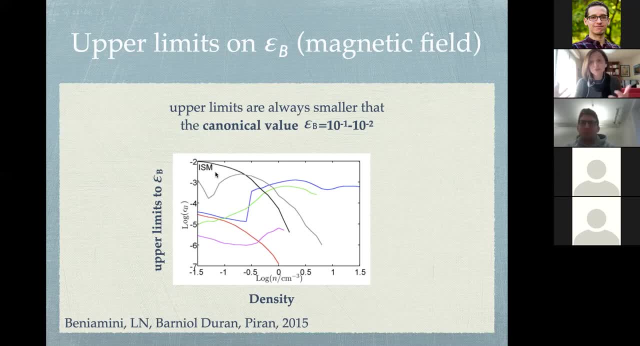 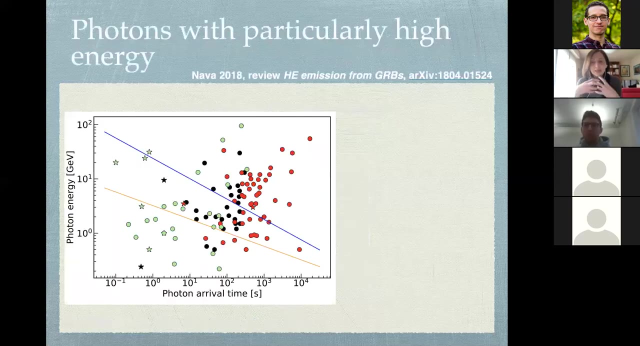 This also suggests that there should be a very high energy component and synchrotron self-compton component at higher energies, because we are lowering the energy density of the magnetic field. Okay, so another hint for the presence of a very high energy component, already present in Fermi data. 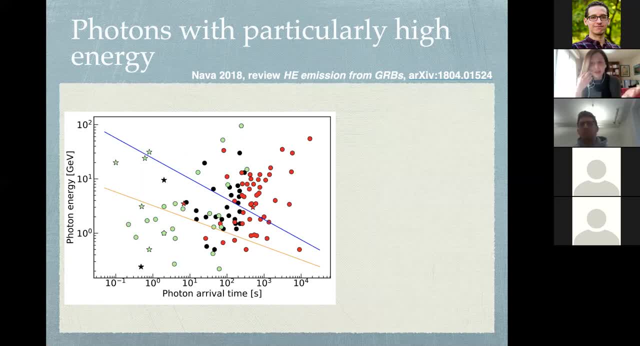 is this one. So this is a plot. I made this exercise in this review about high energy emission from 2018.. So from each gamma-ray burst detected by LAT, I took one photon, just a photon, with the highest energy. So each point in this plot. 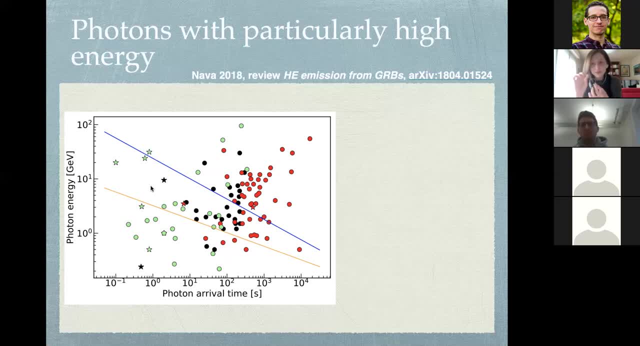 is a photon from a single GRB, It's the one with the highest energy and I plot the energy versus the arrival time. So there is a limit to the maximum energy of synchrotron photons because electrons will be accelerated in the shock to a maximum Lorentz factor. 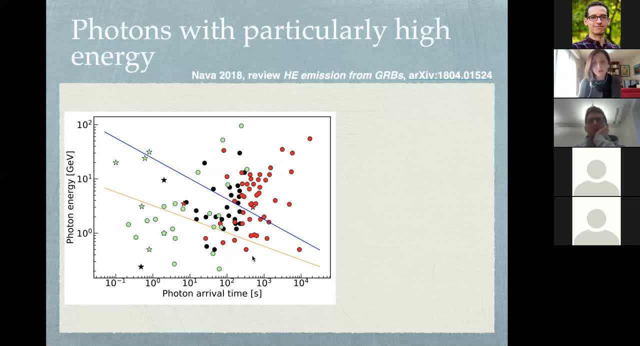 and this reflects into a maximum energy of the synchrotron photons. This maximum energy is in the commuting frame, so in the frame of the fluid is about 100 MeV. It doesn't depend on the magnetic field or any other quantities. 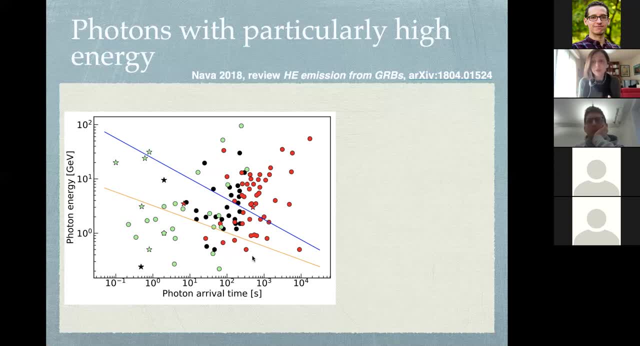 It's a fixed value. if we assume maximum efficiency in the acceleration, so at the BOM rate, So under this assumption, you can derive the very highest possible energy for the synchrotron photons. And then, since gamma rebirths are relativistic, 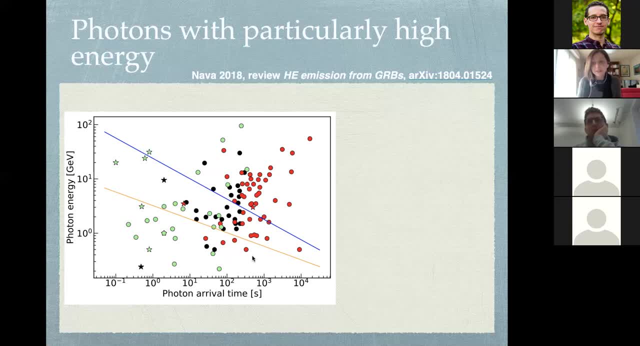 we need to multiply this 100 MeV by gamma, the bulk Lorentz factor, to account for beaming effect. Okay, but the bulk Lorentz factor during the afterglow phase is decreasing because the fiber is decelerating. 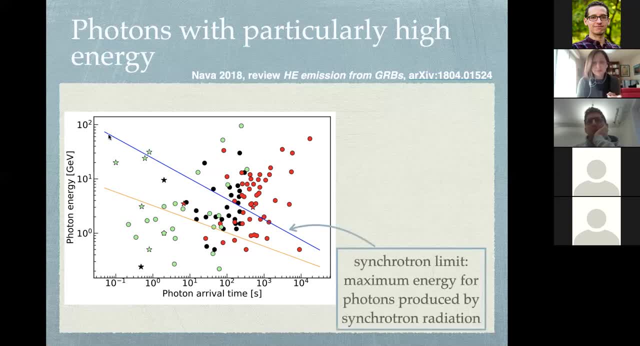 So also this maximum photon energy of synchrotron radiation is decreasing with time. So here I use different assumptions, homogeneous medium, wind-like medium, by playing a bit with the parameters, trying to obtain the highest possible maximum value of the synchrotron photons. 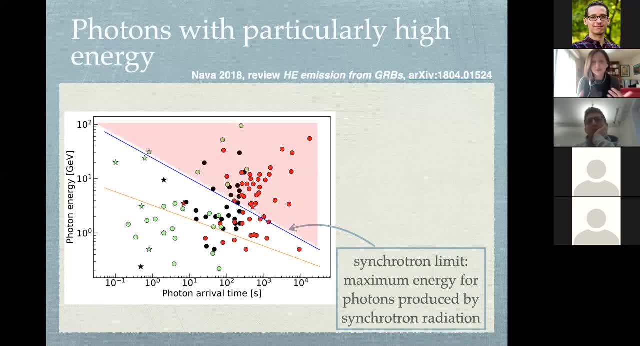 And still, as you can see, there are many photons above these limiting curves. So it's clear that photons above 10 MeV detected after 1000 seconds are almost impossible to explain with synchrotron emission, unless we completely decide that we didn't understand anything. 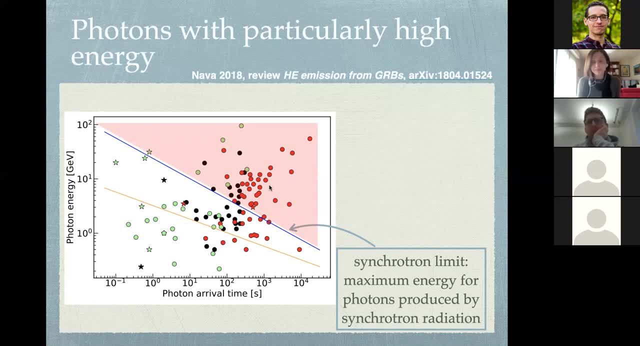 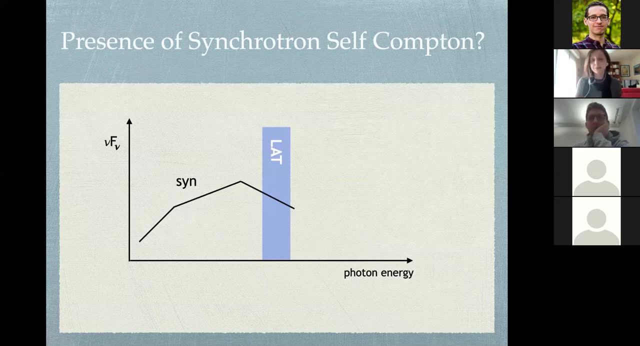 about the acceleration process. So there is in the LAT data a hint for an inverse component. So probably what is going on is that LAT is detecting the high energy part of the synchrotron spectrum, but in the highest part. 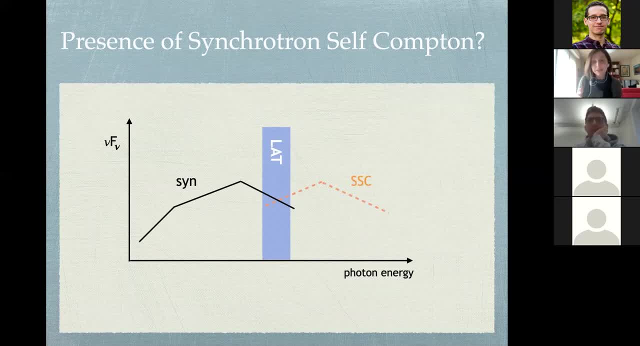 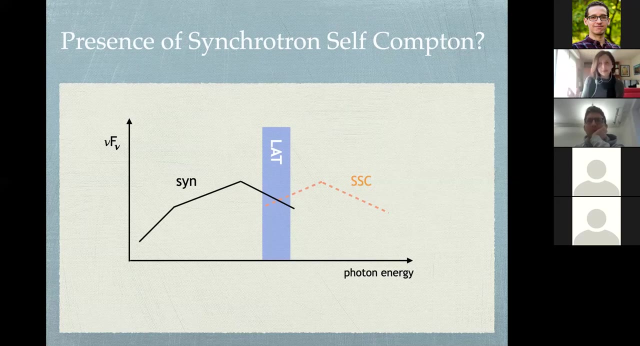 of the sensitivity range of LAT, we see already some photons from a component that is dominating the emission at higher energies. So until a few years ago, the situation was this one: There was the idea that a self-contained component was there, but there was no direct evidence. 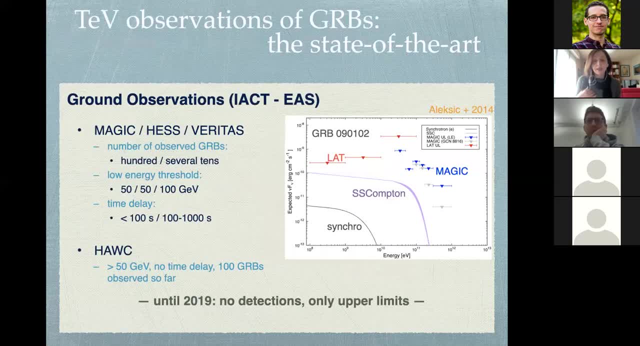 And TV observations until 2019 resulted only in upper limits, so there were no detections. All these ground-based Cherenkov telescopes keep observing gamma-ray bursts, so they observed in the last 15 years 100 gamma-ray bursts with no results. 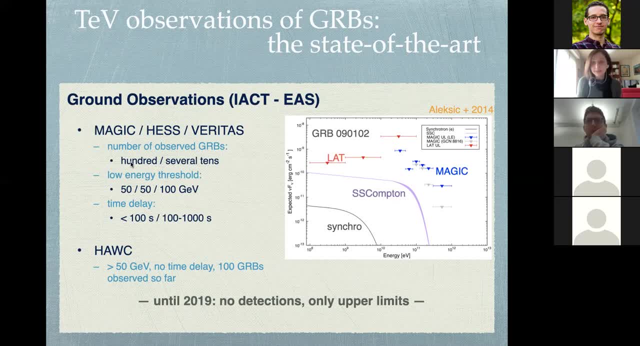 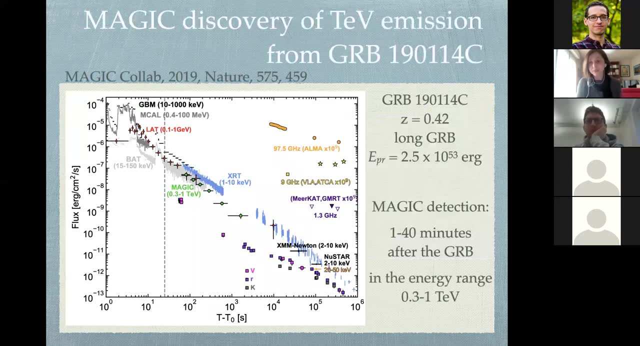 Then, at the beginning of 2019, MAGIC finally announced the detection at TV energies of the first gamma-ray burst. So this burst is called 1901-14C, so detected in January 2019.. Redshift is 0.42.. 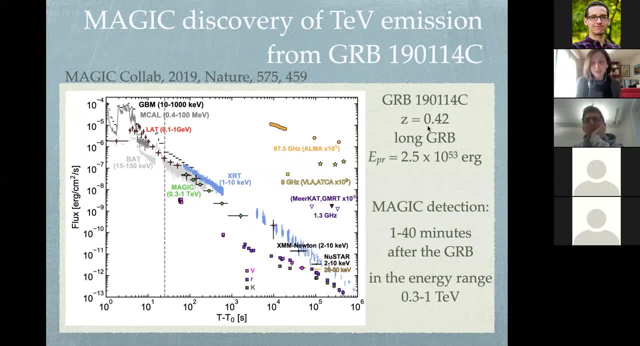 That is quite interesting because at this redshift the absorption of TV radiation from the extragalactic background light is already important. So to detect a gamma-ray burst at one TV from redshift 0.42, it means that intrinsically 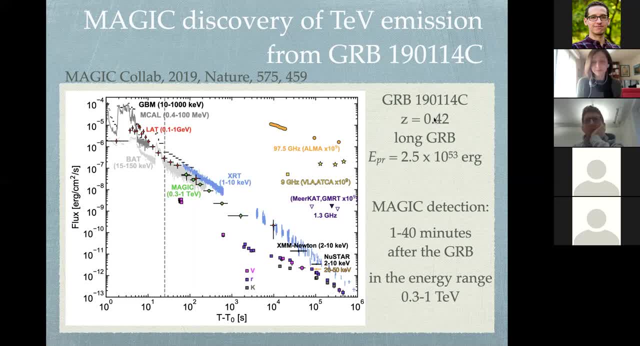 the emission at TV energies was very bright. This is a longer gamma-ray burst. You can see here the prompt light curves. So these are the light curves at all different wavelengths. Here in gray you can see the prompt emission- Prompt emission. 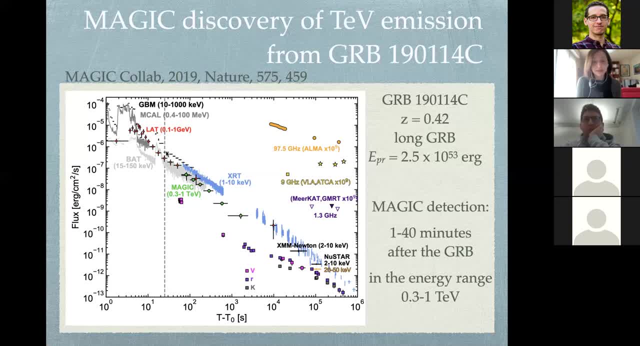 lasts about 25 seconds And then we start to see the afterglow radiation And this is the MAGIC light curve. So this is the first light curve of a gamma-ray burst at TV energies In particular. this is integrated from 0.3 to 1 TV. 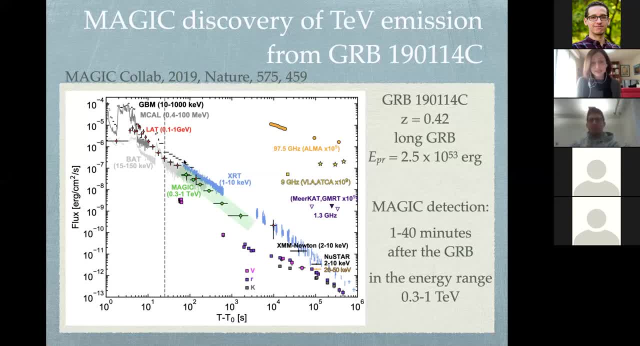 As you can see, it's very similar to the X-ray light curve, So it gets in time as a power law. The energy output in the MAGIC energy range is very similar to the one in the X-ray range and to the one in the GV range. 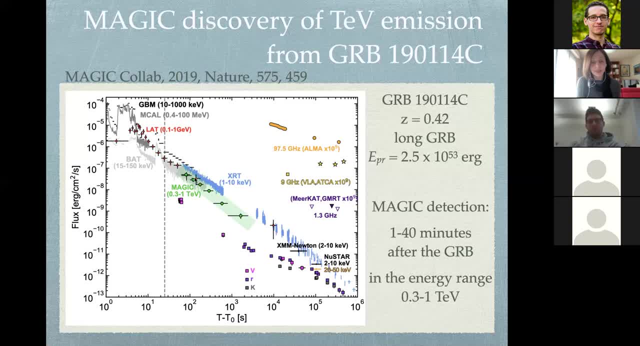 These red points are the emission detected by LUT. LUT could not observe from here to almost 10, to the fourth seconds, due to observing constraints, And then, when the gamma-ray burst entered again the field of view of LUT, LUT detected again. 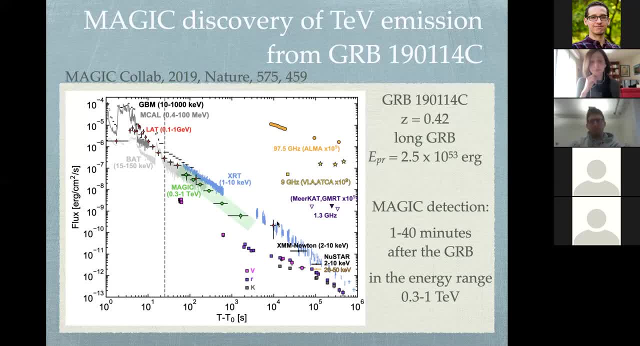 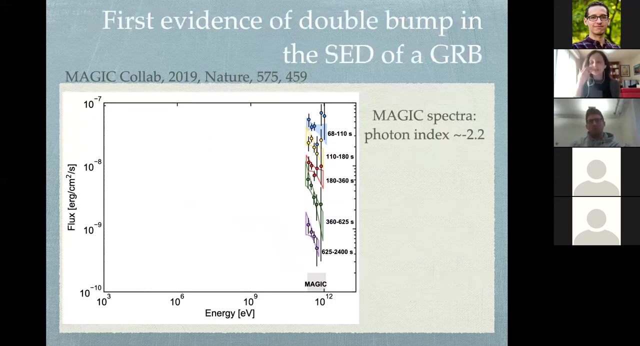 a GV emission from this gamma-ray burst. Okay, So MAGIC started observation one minute after the prompt emission, So it was very quick in pointing the gamma-ray burst and observed significant emission up to 40 minutes after the gamma-ray burst. These are the spectra. 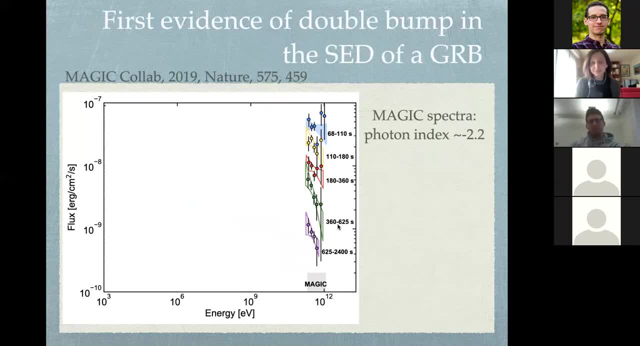 by MAGIC in different energy ranges, sorry, in different time intervals. So the photon index probably evolves with time, becomes softer at later times, but it's always consistent within the errors with minus 2.2.. And for the first two time intervals: 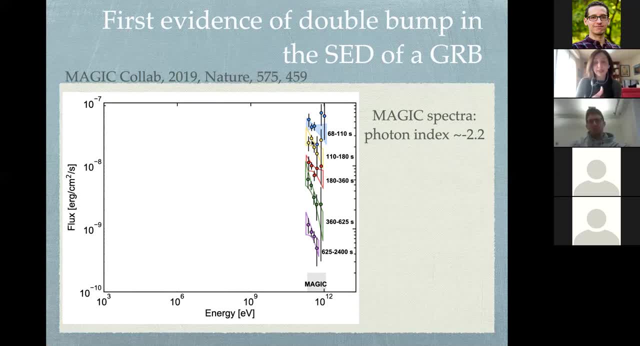 we can compare the SED. so we can add in this plot also BAT, GBM and XRT data. So this is the comparison between X-rays and the very high energy range And, as you can see, the amount of energy. 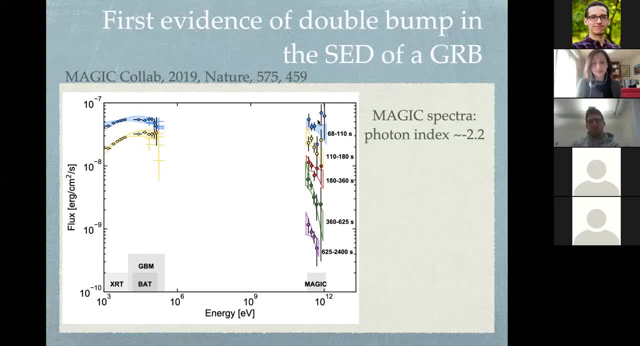 is more or less the same in two different energy ranges, And here LUT observations were fundamental to show that there is actually we are looking at two different spectra components, because if you add LUT data, you can see that clearly there is a double bump. 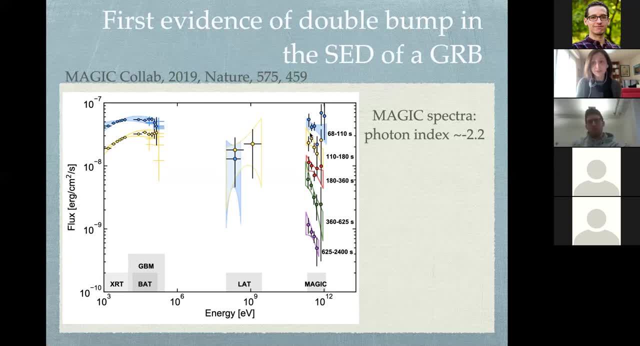 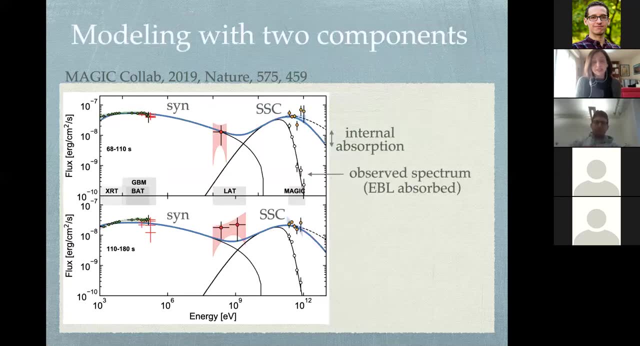 in the SED of gamma-rebursed. So this is the first evidence for a double bump in the SED of gamma-rebursed. So in the MAGIC paper we propose modeling of these observations as synchrotron plus synchrotron. 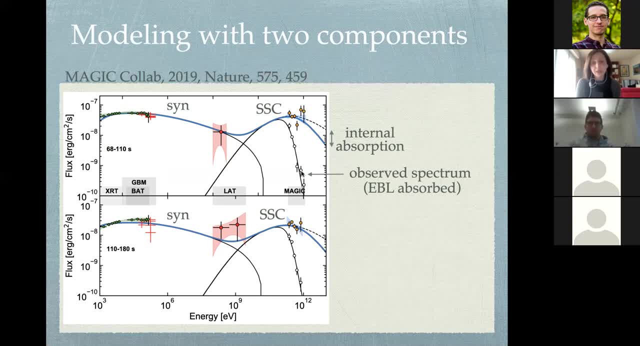 self-content component. Of course we need to model not only the spectra at some particular time but we need, with the same model and same parameters, to explain also all the temporal evolution. So model the light curve at different frequencies. So you see here. 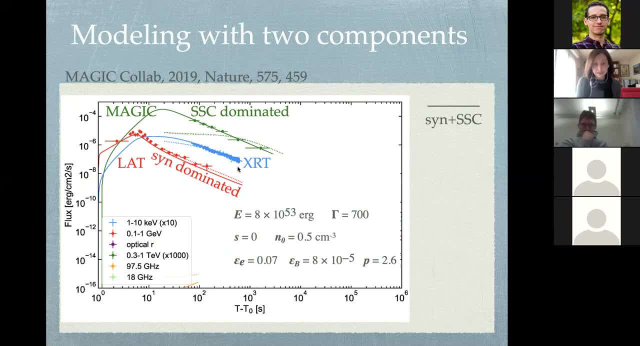 the light curves by MAGIC, XRT and LUT and with the solid line, the modeling, that is already the sum of the synchrotron plus SSE component. MAGIC, of course, is always dominated by the SSE, LUT is dominated. 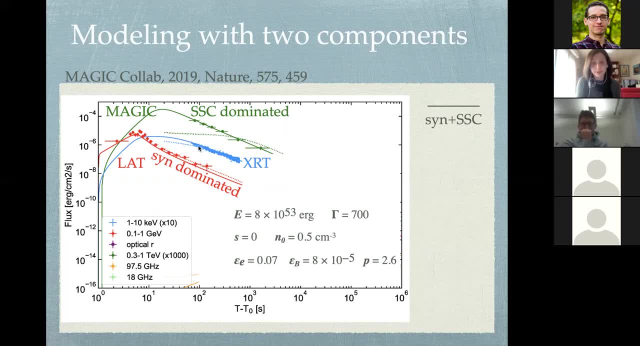 by the synchrotron emission And of course also XRT is always dominated by synchrotron. These are the parameters that we infer. So there are the values of the parameters that we infer from the modeling. So the energy is quite large. 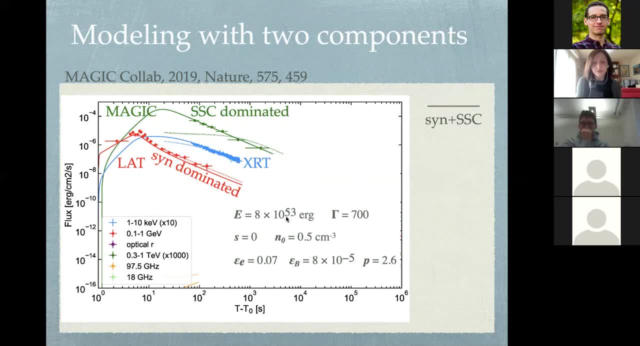 It's larger than what emitted during the prompt, a factor of two or three. The Lorentz factor. in the initial Lorentz factor of the fireball it's around 700.. And here you can see the other parameter, Epsilon B. 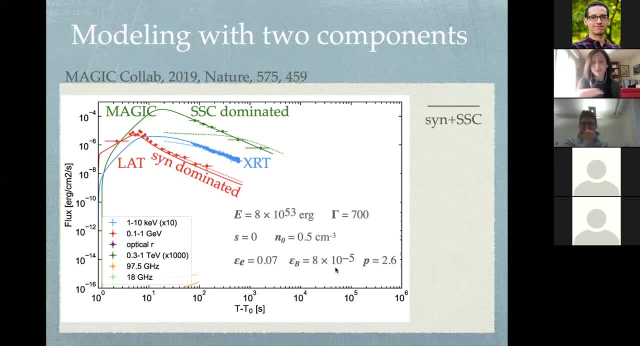 as already inferred from GEV data alone is quite small, So 10 to the minus four, While the fraction of dissipate shock, dissipated energy that goes into the electrons, is 7%, So consistent with the usual assumption of 10%. 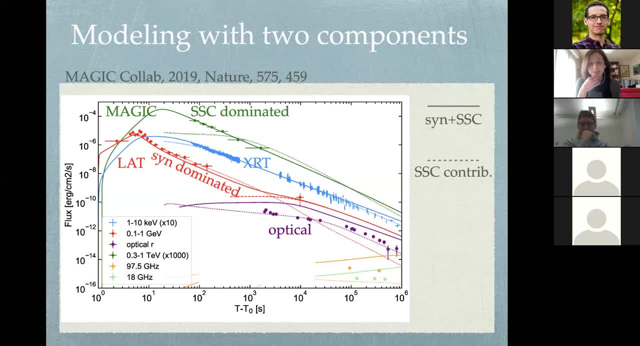 If we go a later times there is something very interesting. So first of all, you see that this LUT detection at 10 to the fourth seconds is now dominated by the synchrotron self-quantum contribution. So here I'm plotting explicitly: 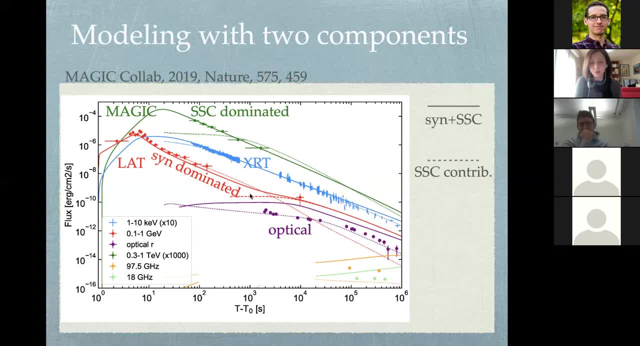 the flux of the SSE component And, as you can see, this last point is inverse quantum emission. So it means that synchrotron and inverse quantum are shifting to lower frequencies, And now the SSE enters the LUT energy range. 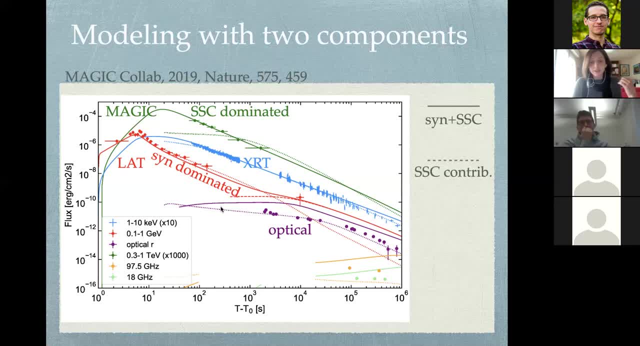 Okay, There are a few problems. I'm not sure I can comment deeply in all of them, but, as you can see, optical data are not modeled by this very same model that is able to explain early time emissions, So this might point to an evolution. 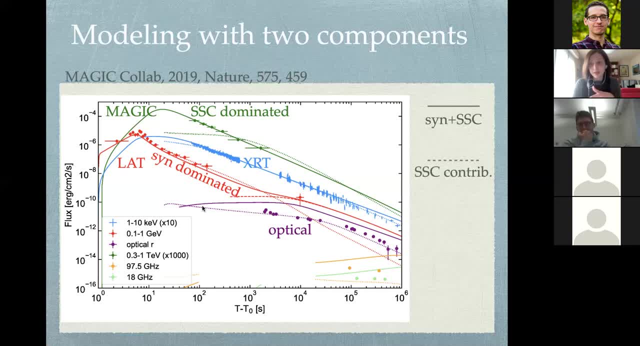 in time of some parameters. We always assume in gamma-reversed after-world modeling that the efficiency for accelerating the particle, for amplifying the magnetic field, are always constant in time, even though the fireball is accelerating and becoming at some point even non-relativistic. 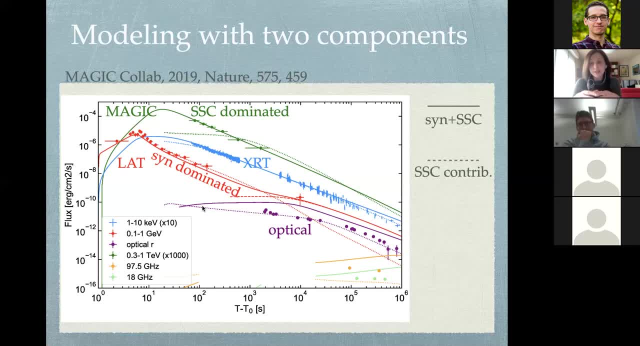 So there are a few problems. This might be an indication for the fact that the picture is more complicated and we need to start invoking some evolution in time of the parameters. The dotted line shows a different modeling that optimizes the modeling at late times. 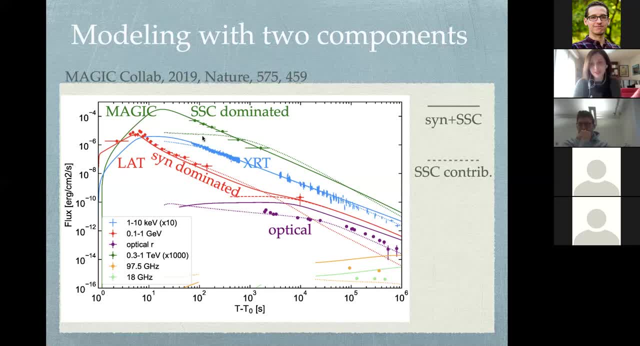 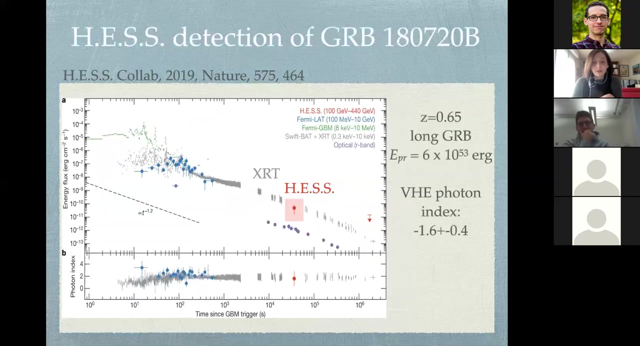 but it's inconsistent with early time magic observations. So this might be an indication that some parameters may evolve. in particular, the efficiency for shock acceleration and magnetic field amplification may evolve with time. Okay, then there was another announcement for a detection. 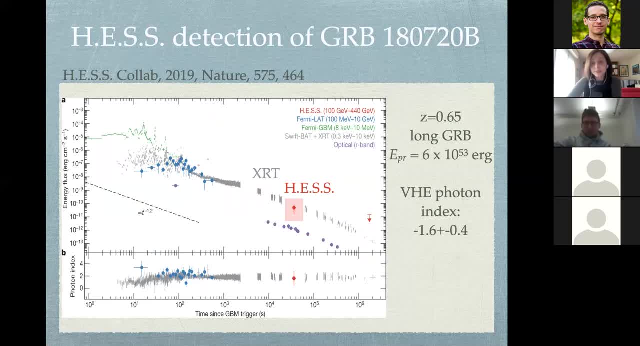 of TV radiation from a gamma-reversed. So this gamma-reversed was from 2018, but, as announced, the detection only after the detection by magic. So in this case we have only one point, so there is no light curve. 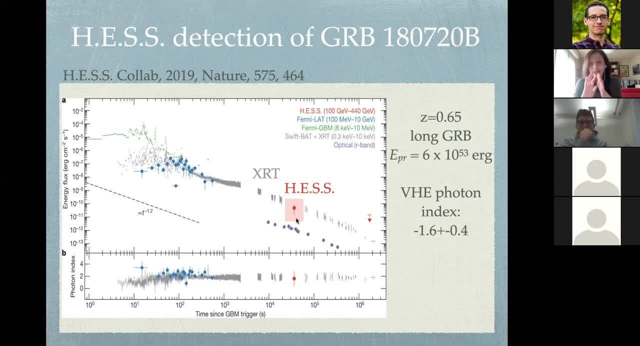 but there is one detection at around 10, 11 hours after the prompt, so at much longer time. as compared to the magic detection, This gamma-reversed is at even higher redshift. so 0.65, still a long gamma-reversed. 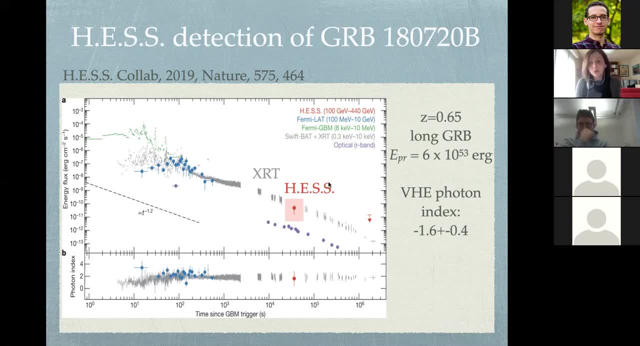 and what is very interesting here is that also in this case, the TV flux- actually this point- is integrated between 100 GV and 440 GV, So in this energy range the luminosity that we see is again similar to the luminosity emitted. 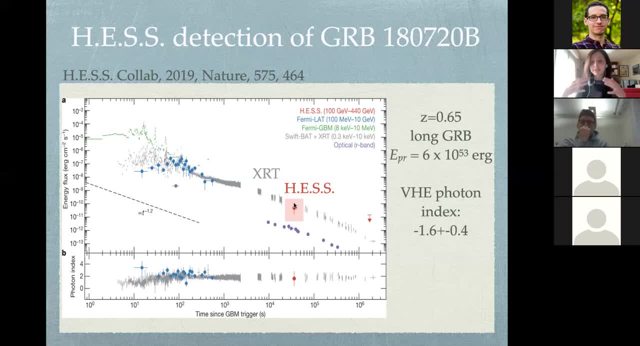 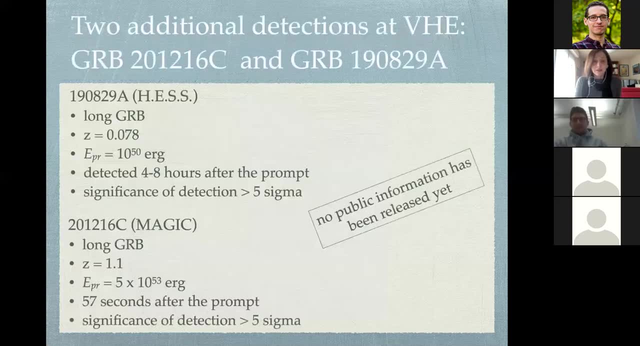 in the X-ray energy range. This means that synchrotron and inverse quantum component share a similar amount of energy. Then there are two additional detections at very high energies, one by S and one by magic. However, there is no public information yet. 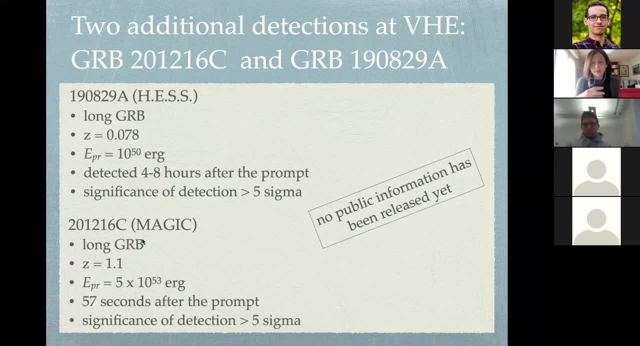 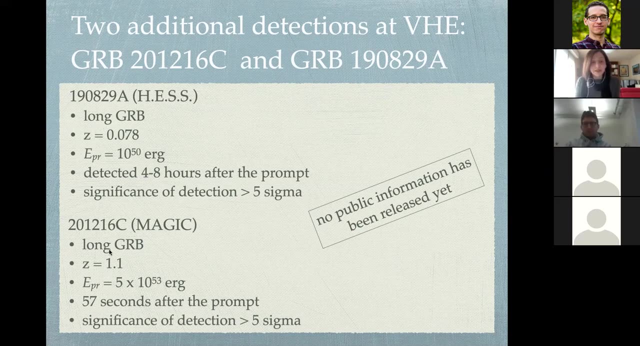 on these two detections only. what the collaborations I have released in the GCN archive that these are short telegrams to inform the community about the detection. So again, in both cases these are long gamma-reversed. In the S-detected gamma-reversed 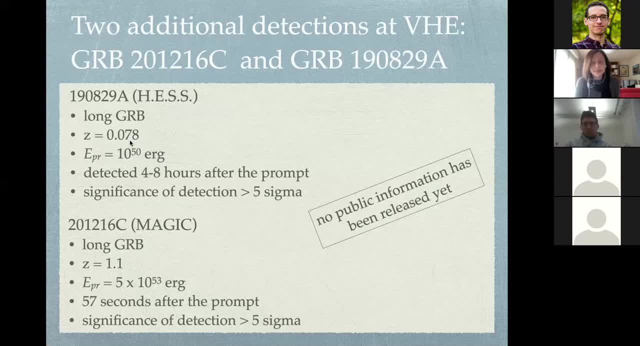 the redshift is very small: 0.078.. The gamma-reversed is not particularly energetic, so we learn that it's not necessary to be very bright gamma-reversed in order to produce this TEV component. But, of course, if the gamma-reversed 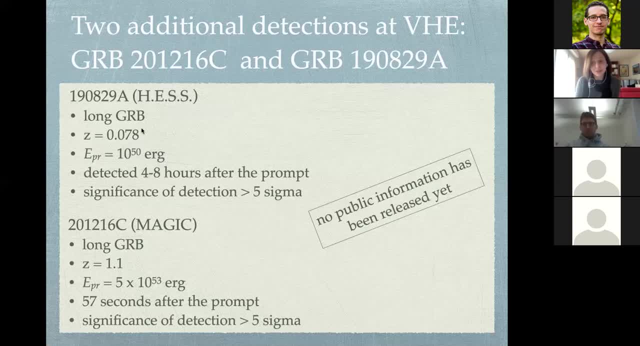 is not very energetic, it needs to be nearby in order to detect the emission. The radiation was detected four to eight hours after the prompt and the detection is significant and more than five sigma. This is all the information we have so far For the magic gamma-reversed. 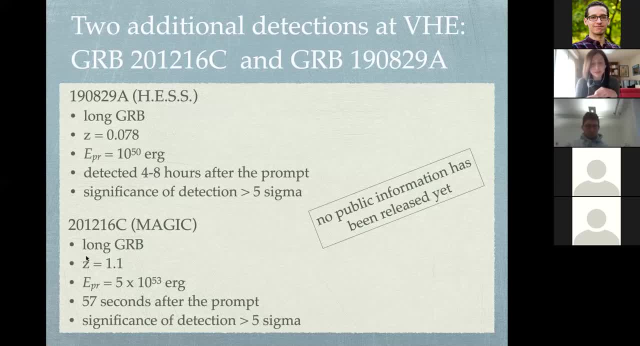 what is particularly interesting is the redshift. So this time magic detected this gamma-reversed at redshift 1.1, which is very, very large. So this is very promising also for future detection with CTA, because it means that we can really detect gamma-reversed. 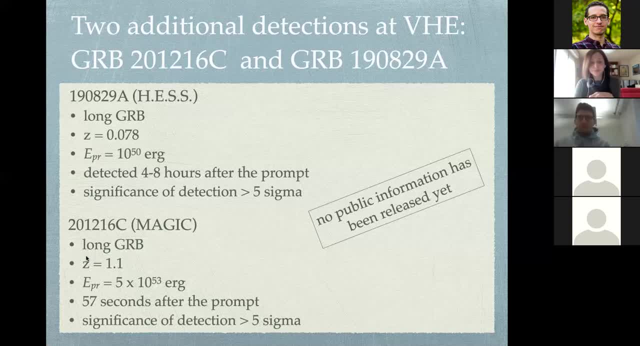 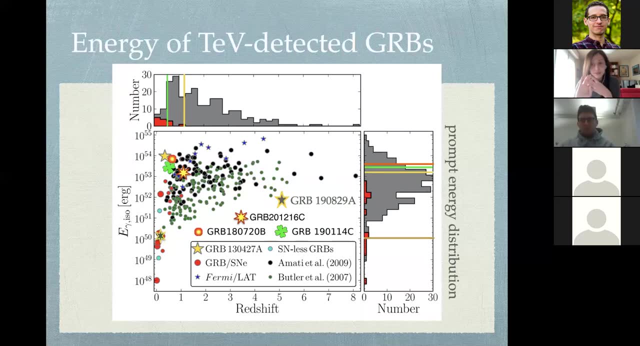 even when the redshift is quite large. This is a summary of the properties of these four gamma-reversed. These are the gamma-reversed detected so far by Cherenkov telescopes. So you see here: distribution of population of gamma-reversed in the plane, prompt energy. 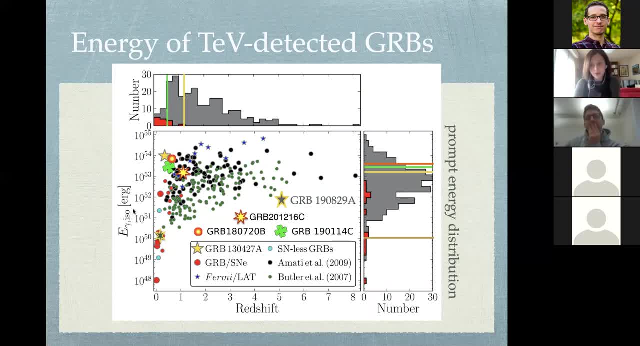 So this E gamma I is the energy emitted during the prompt versus the redshift, And so all the gamma-reversed detected by Cherenkov telescopes are here, of course, with quite large energetics and redshift smaller than one. Plus there is this subluminous. 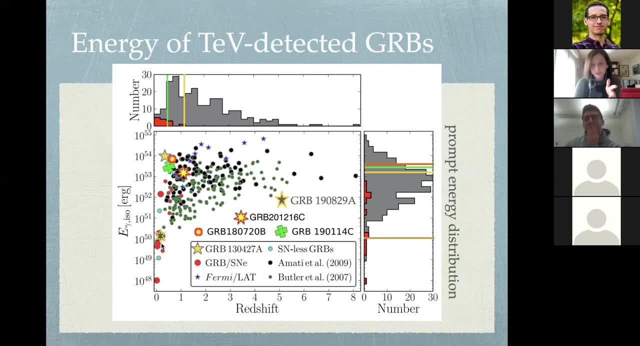 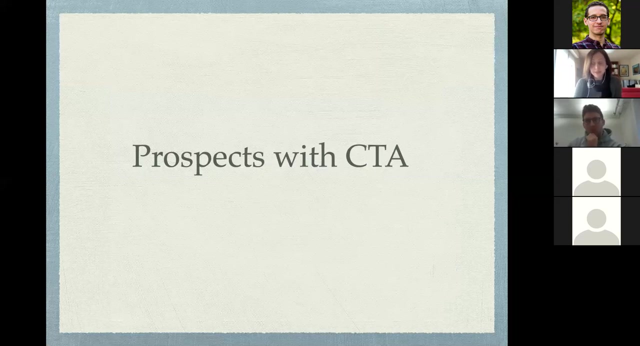 gamma-reversed detected by S at very small redshift. OK, so this gives an idea of how this small population of TV-detected gamma-reversed compares with the full population, at least in this plane. I would like to conclude mentioning a bit the prospect. 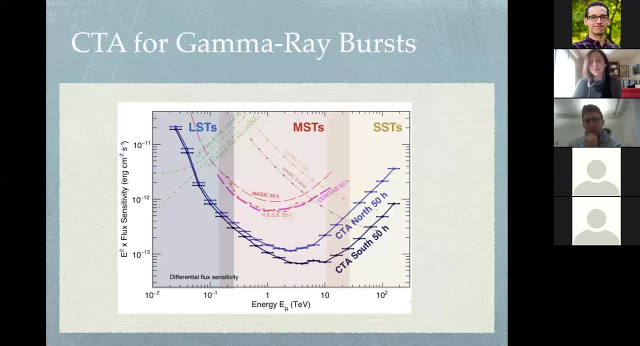 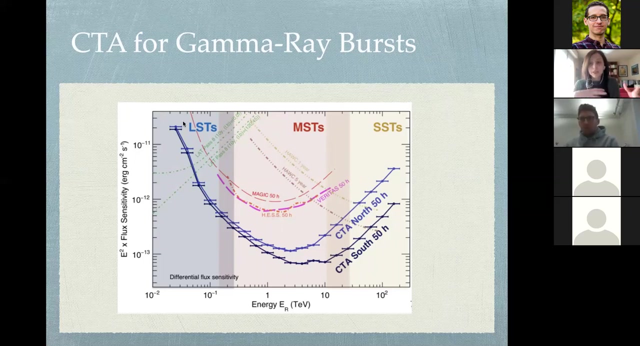 for CTA. So the Cherenkov telescope array will have three different telescopes, The LST, so large size telescopes that are sensitive in this low energy range. So in particular they will be sensitive down to sorry, down to 20,. 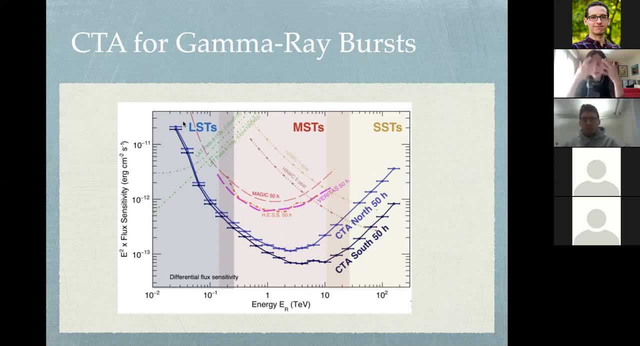 30 GV. That is particularly relevant for gamma-reversed, because at these energies the emission is not attenuated by EDL, also at high redshift. And then we have the MST medium-sized telescope that will be sensitive at higher energies. 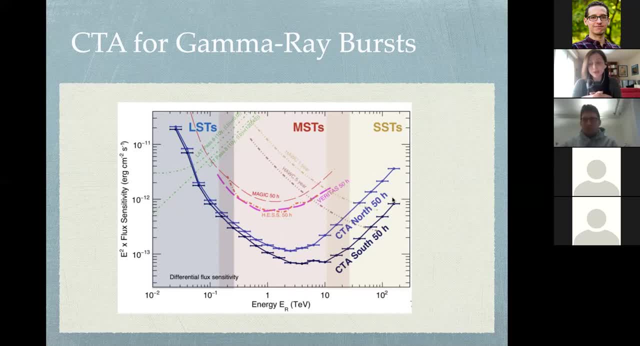 We do not expect to have useful information from the small-sized telescopes that are sensitive above the NTV, where it's really really difficult to measure emission from a gamma-reverse due to strong EDL attenuation. But for sure, with the information. 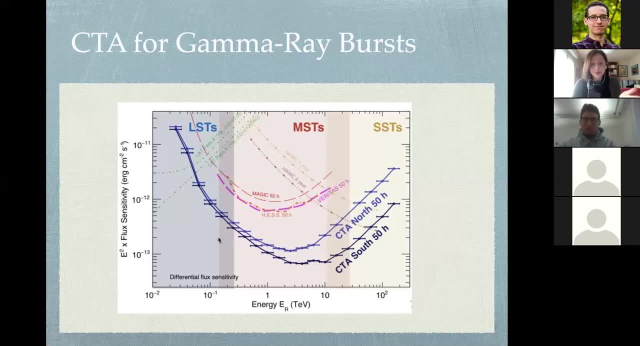 that we have so far from this recent detection. we know that the LST and MST will play a very important role in increasing the number of gamma-reverse detected at these energies. Here there is a comparison with the sensitivity of MAGIC and ESSEN. 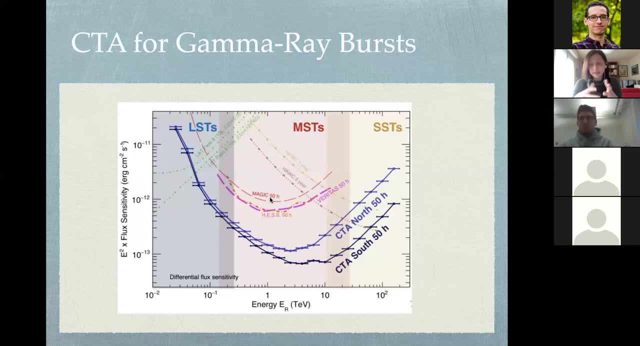 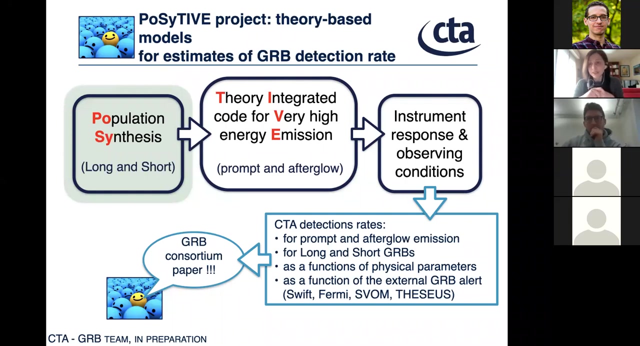 So this plot gives an idea of the fact that we will really change and improve our TEV view of gamma-reverse with the CTA. There is an ongoing effort in the CTA collaboration to try to estimate the detection rate and also try to understand. 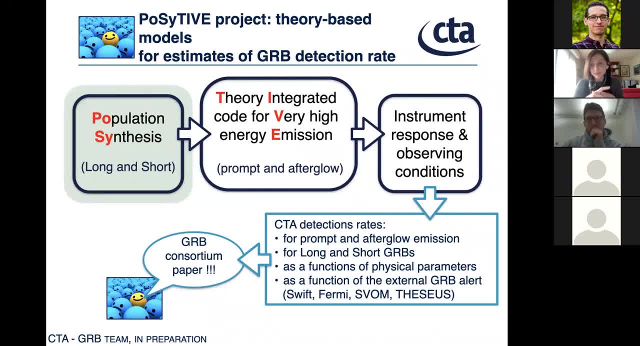 what is the gamma-reverse population? that will be accessible with CTA, And so we are using population models for gamma-reverse starting from an intrinsic population that is consistent with what we see and what we detected- 1,000 gamma-reverse detected so far. 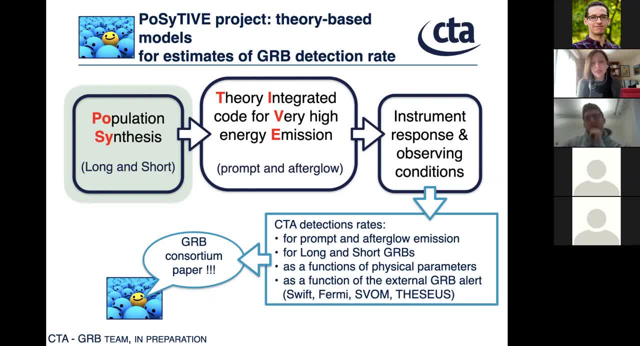 in the soft gamma-ray range. And then we are modeling both prompt and afterglow radiation at very high energies, based on theoretical models. for the afterglow Now we also have observations that support the modeling, And then we will perform simulations of the CTA. 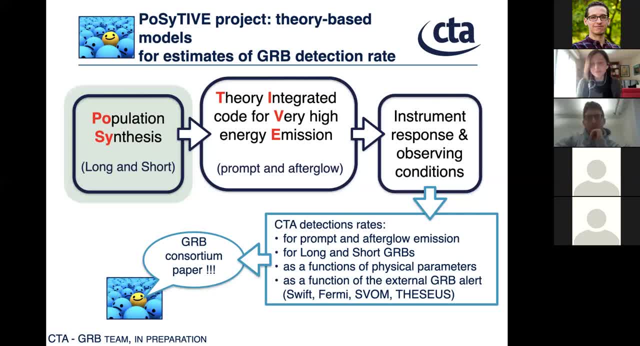 how CTA will respond to this predicted TEV emission and its evolution time, And so a consortium paper is in preparation where we investigate quite in detail how CTA will be able to detect- prompt, hopefully- and afterglow radiation from short and long gamma-reverse. 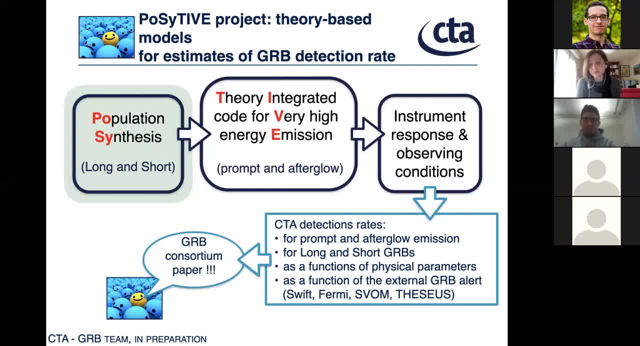 There is also a study that is investigating synergies with detecting interferometers for gravitational wave detectors and also synergies with next generation of emissions for the study of gamma-reverse, like SWAM or TCUs, And so preliminary results are very encouraging because we are estimating. 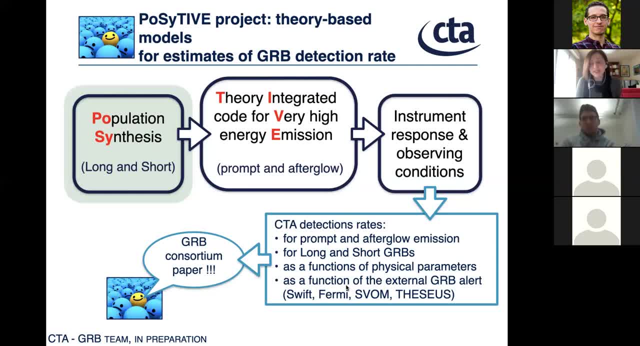 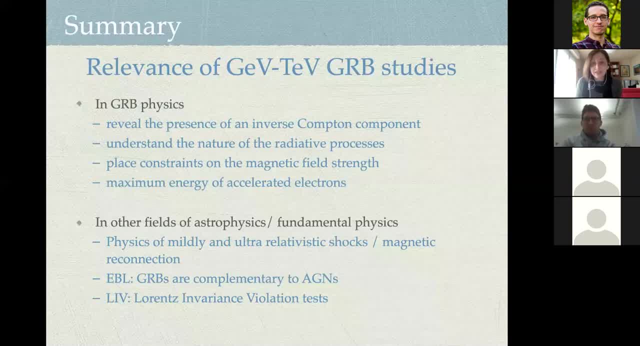 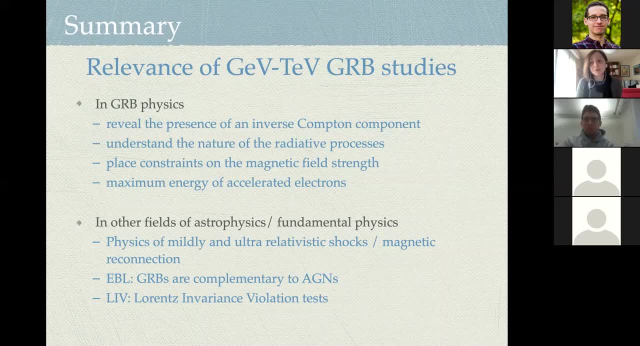 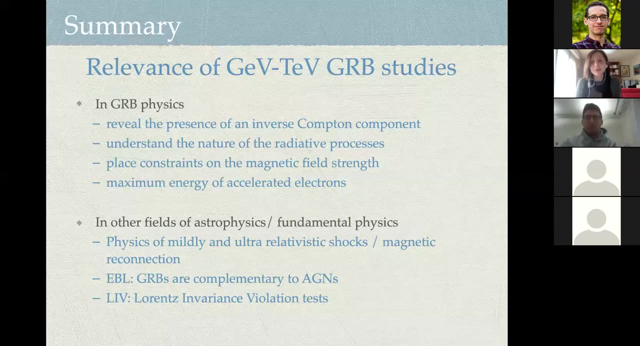 from a few to several gamma-reverse detected by CTA per year. So this will really change our understanding of the phenomenon and add information to the general picture. So to summarize why it's relevant to have GEV-TEV observation for gamma-reverse studies. 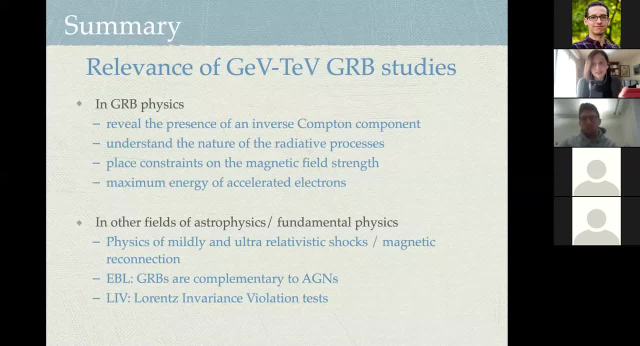 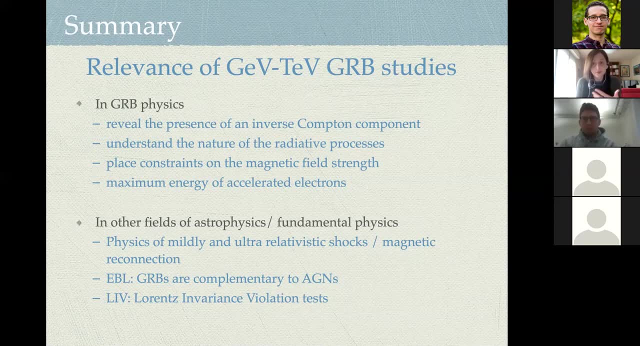 Well, first of all, GEV, together with TEV radiation, reveal the clear presence of an additional component, probably inverse content, And we can better understand the nature of radiative processes. So the next step is try to detect TEV radiation from the prompt emission. 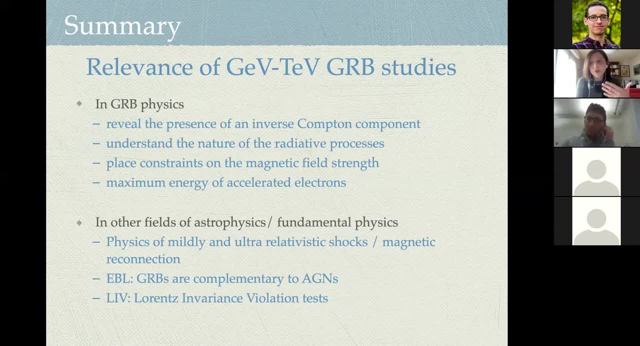 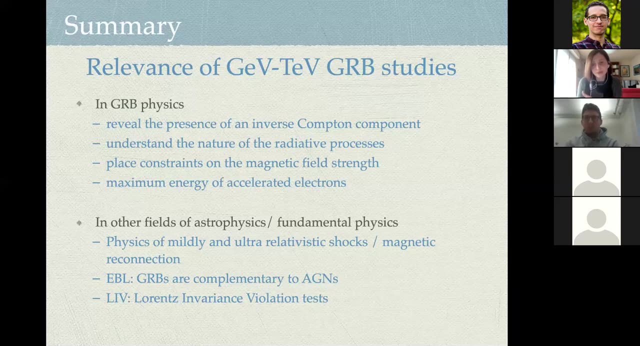 of gamma-reverse, where we really don't know what is the nature of the sink of the prompt emission detected in thousands of gamma-reverse. We still have no clue about the origin of this radiation. So to understand what's going on at TEV energies, 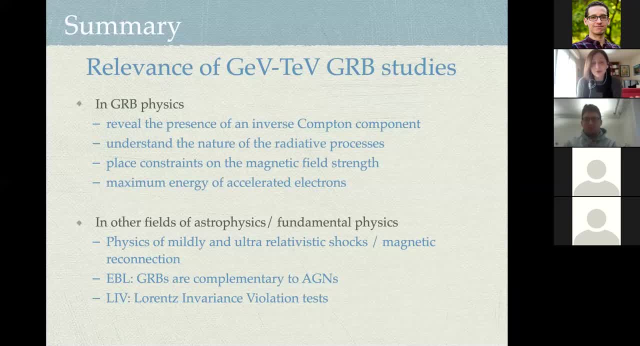 might help to understand the nature of the heart X-ray component. And then we saw how we can place constraints on the strength of the bioenergy field. by measuring the relative importance of synchrotron versus inverse-compton component, We can put a limit. 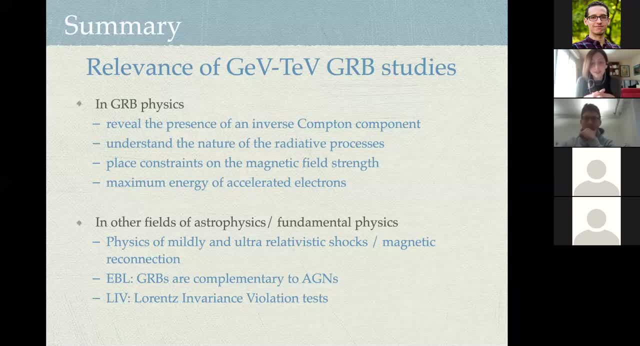 with GEV observation to the maximum energy of the accelerated electron In general. let me mention just to conclude that these studies can be important also in other fields and not only in gamma-reverse physics. We can understand better physics of mildly and ultra-relativistic shocks. 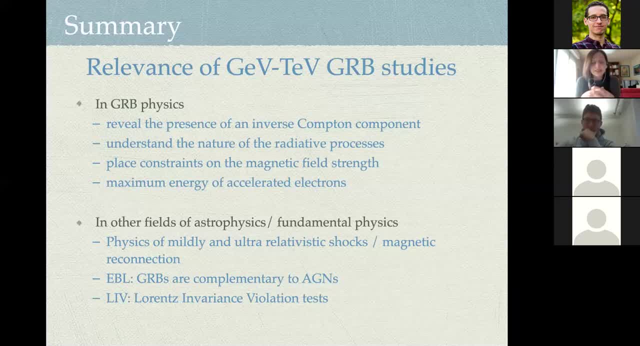 or magnetic reconnection, And these observations have been already applied to study EBL studies. So gamma-reverse can be complementary to other sources to constrain model for the EBL, the extra-galactic background light, And especially important is the recent detection. 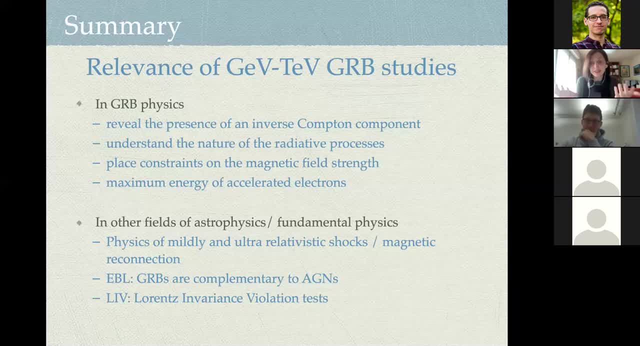 of gamma-reverse at TEV energies at red chip 1.1.. So we can really extend to relativity, large red shape, the study of EBL with a complementary source and, of course, test for Lorentz invariance null violation. So I will stop here. 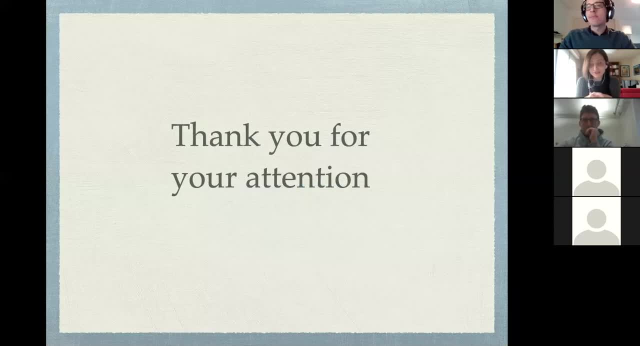 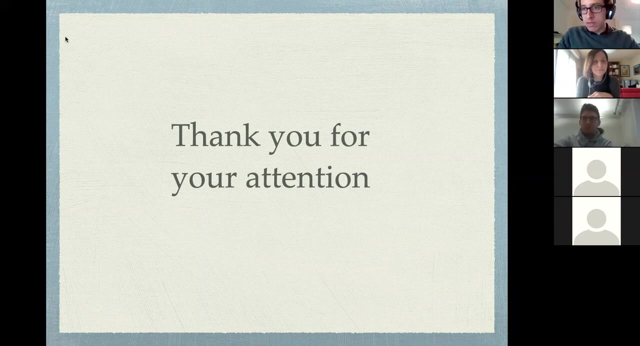 and thank you for your attention. Thank you very much, Laura. It was a very, very nice overview of GRBs. Is there any question already in the audience? You can just raise your hand or unmute yourself and ask right away. I think Tom has a question. 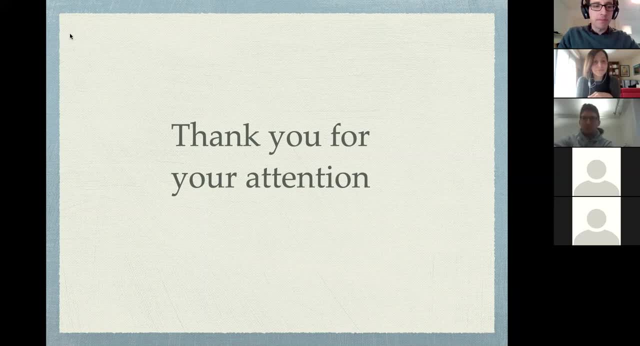 Go ahead. Yeah, just two quick ones if that's okay. The first was, unless I missed something, it looked like the TEV emission was often after the prompt. Is that correct that the emission seems to be the TEV as part of the afterglow emission? 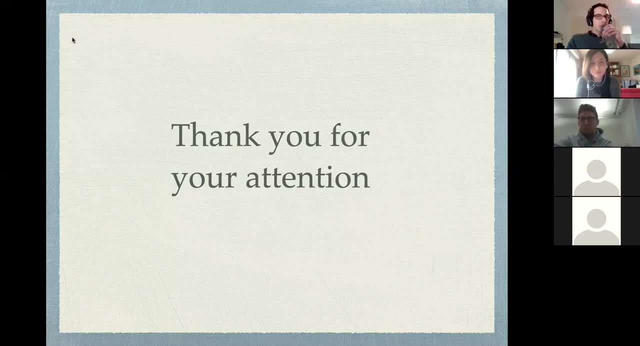 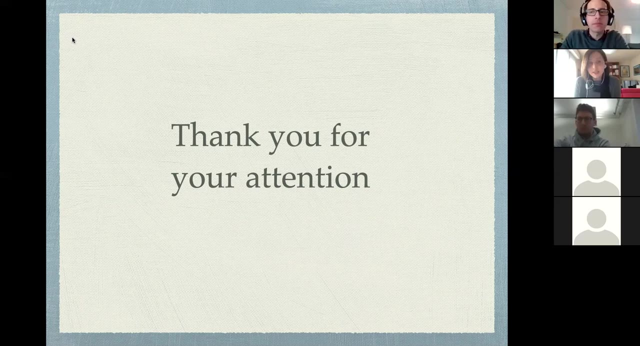 or is that just something kind of observational? So the field of view of the stirring of telescopes is of a few degrees, So they need an external alert, So from a flight like Fermi or SWIFT that provides the exact location of the GRBs. 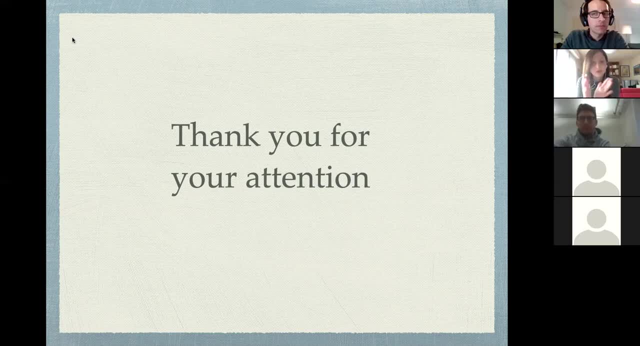 and then the telescope will point the circle. It needs time to move and point and place the GRBs within the field of view. MAGIC is particularly suited for this because it can move and point the source in 30 seconds. It depends, of course. 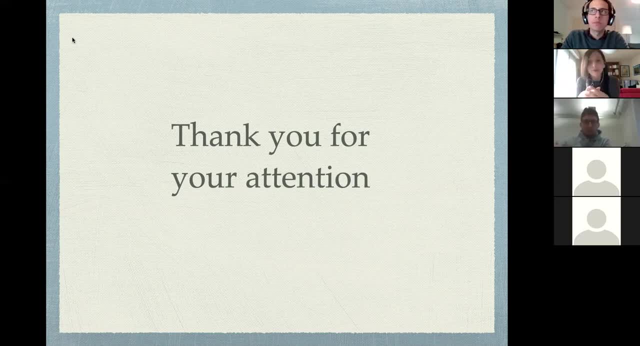 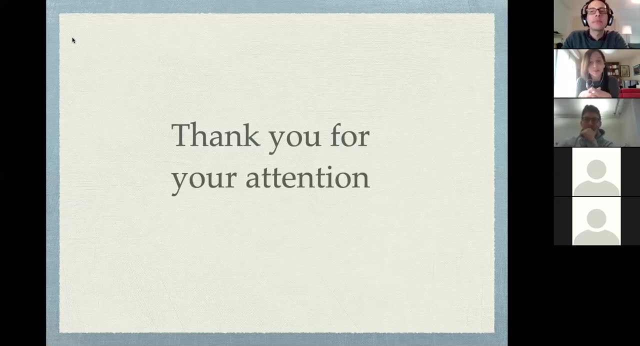 on the initial position of the telescope and the final one. But there is also one case in which the camera reverse was pointed 24 seconds after the prompt emission. So far there is no evidence of TEV emission during the prompt. No evidence, There is no. 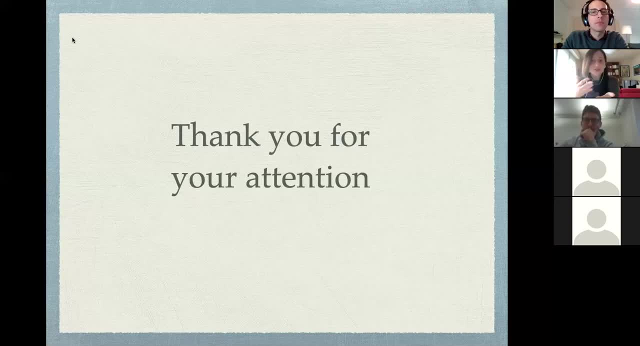 We never were able to start observation when the prompt emission was still ongoing. So we need a combination of particularly long gamma reverse, or maybe lasting hundreds of seconds, and a very faster pointing. So so far it's only after glow radiation because no telescope. 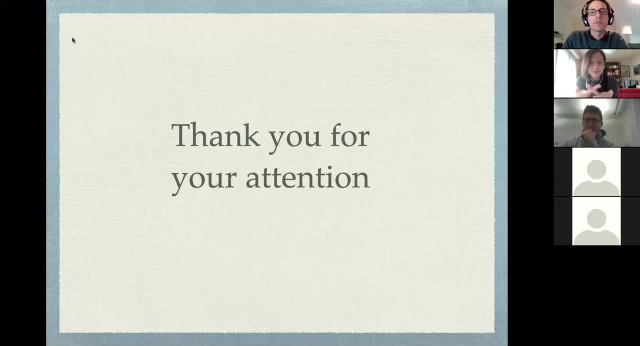 was able to observe the gamma reverse already during the prompt. I see. Thank you very much. The other question I have is just: is there any kind of emission? is there any known source of kind of precursor emission or anything before the prompt? or is prompt really? 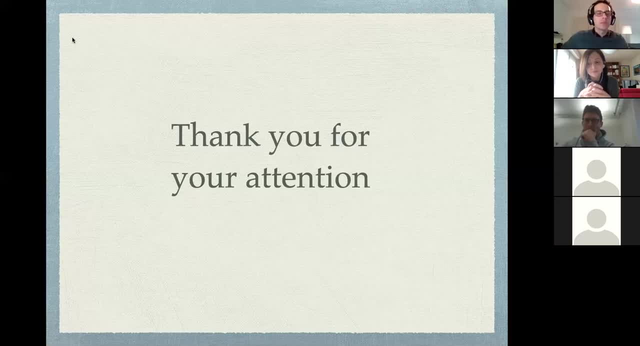 the first place you get the emission. No, but from TEV energies, you mean, Or in general, I guess, high energy, GEV or TEV- Would you expect to see anything before the initial burst? No, So sometimes when you look, 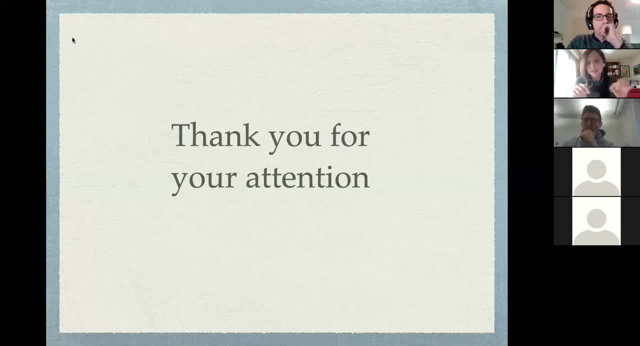 at KEV data, KEV data for ARDAX rays, you can see a precursor- what is called a precursor- sometimes even tens of seconds before the main event. But again at TEV energies it's difficult because the Cherenkov telescope 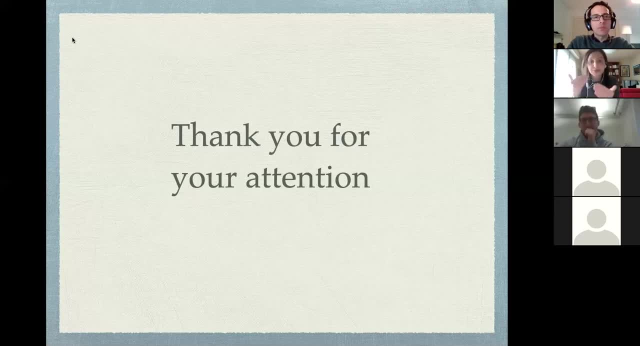 is not observing the gamma reverse before, So you cannot look to previous data and see if you find something. It's not expected. This precursor that we see in ARDAX rays of soft gamma rays are another big puzzle of gamma reverse physics, So we really don't know. 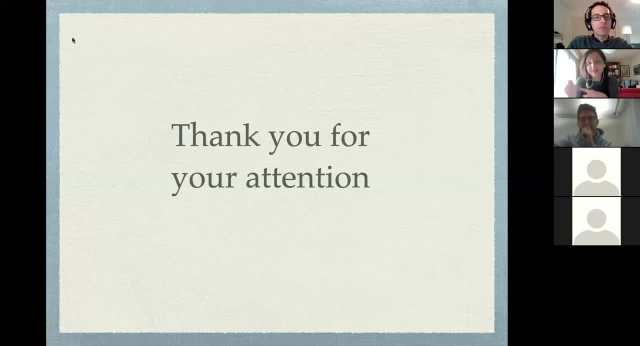 what is going on there. but it's difficult to study the precursor at different wavelengths because usually in optical, in all the other bands, you need to point the source. So you need first the alert from a gamma-ray satellite. I see. Thanks very much. 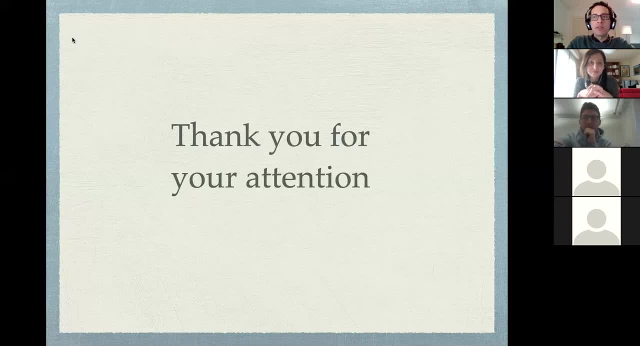 Irene had a question first. Yeah, Thanks for this nice overview. I was wondering when you were mentioning about these most recent observations. you say that to explain them, it would be nice to have a temporal evolution of some of the unknown parameters. 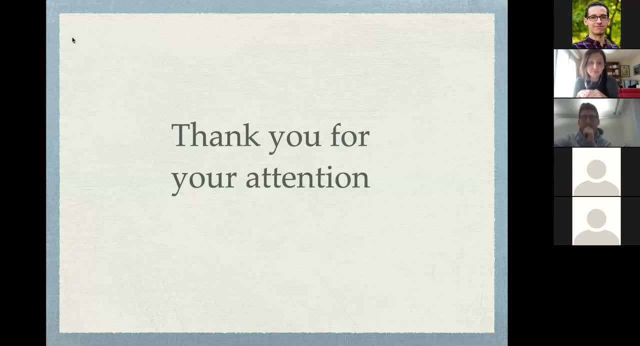 which would be epsilon E and epsilon B, And I was wondering whether you can comment on the prospects of actually learning how they evolve as a function of time, because they are very uncertain now. So what are the prospects of improving these with the CTAS? 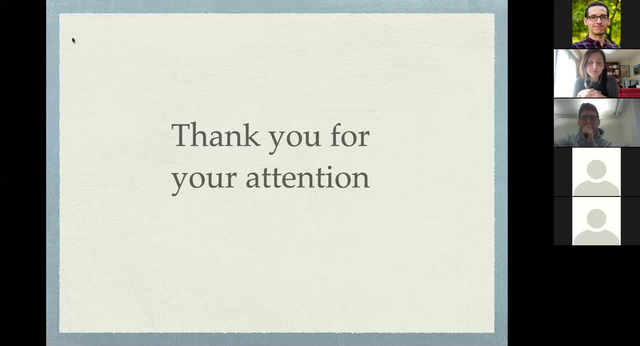 or other facilities. So this evolution of the parameters described in the shock were already proposed before this very energy observation, because very often we are not able to explain X-ray, optical and radio observations. There is always something that it's not easy. So maybe we see a break in the optical 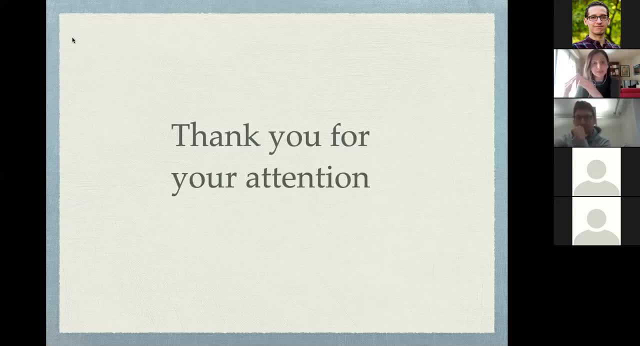 that is due to the fact that a break of the synchrotron spectrum is crossing the optical band, but this is not consistent with what we're seeing in the X-ray. So very often the simple afterglow model, where all these parameters 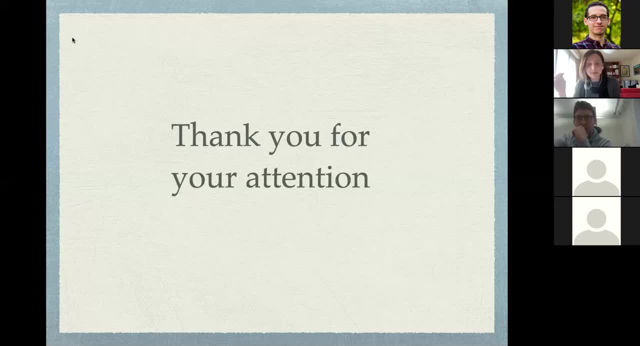 are constant in time, fails in explaining the afterglow radiation. Now we have this additional energy window. that is showing- this is my personal opinion, but it's showing that this model is limited. Even though we have time-free parameters, there is something that is not working. 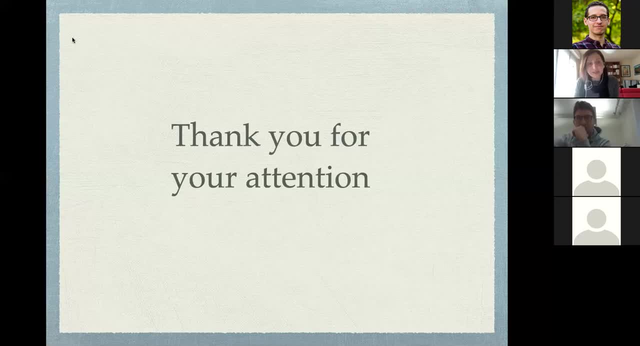 And so, yes, one possibility is to start playing a bit with these parameters. So, of course, if you start to have more and more data at early time and you follow the evolution to late times, you can really start to see a trend, maybe. 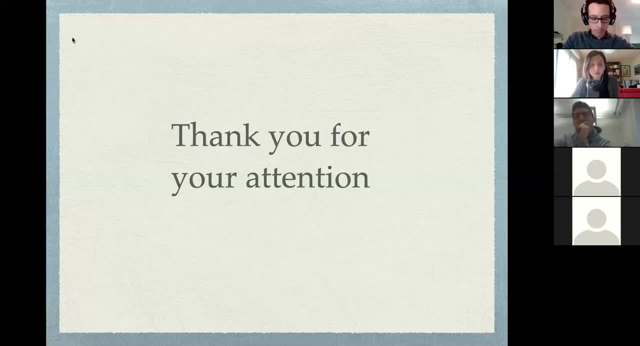 So in old gamma rebirths you need to have one of these parameters that work in time in a certain way So you can start to see something systematic in old gamma rebirths. So this can be a nice investigation to do with more data. 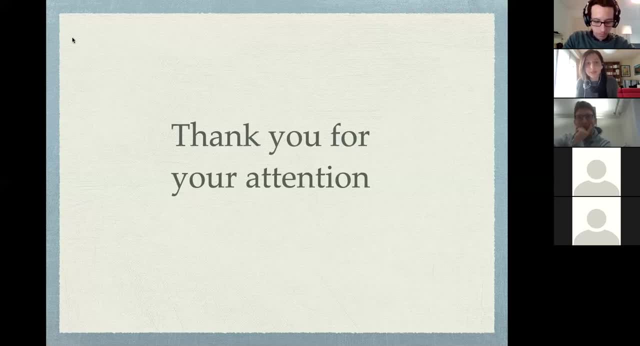 Of course you need well-sampled light curves at different wavelengths, And this is quite rare. So you see, for this gamma rebirth effect at MyMagic, a lot of beautiful data, because Magic announced immediately the detection and then all the facilities started observing. 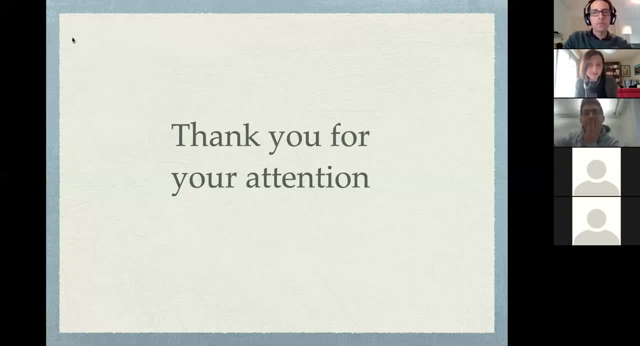 the gamma rebirth, But usually for an average gamma rebirth this is not the case. Okay, thank you, And Luca has a question as well. Yes, Ciao, Lara, Very nice talk, Just a question, Ciao, Luca. 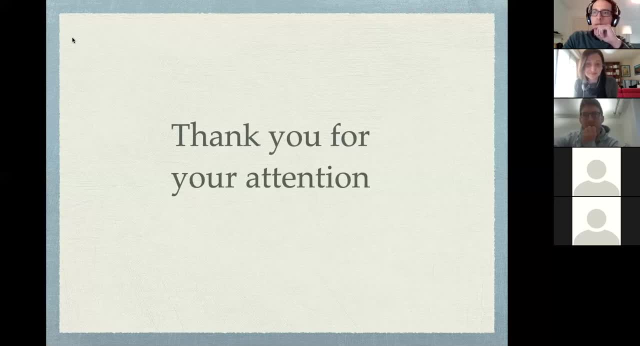 There are some evidence, at least in two of the GRBs that you have presented in your talk, That the local environment is quite dense, and the evidence comes from the high extinction found along the line of sight. If I understand correctly, this TV component is mostly associated. 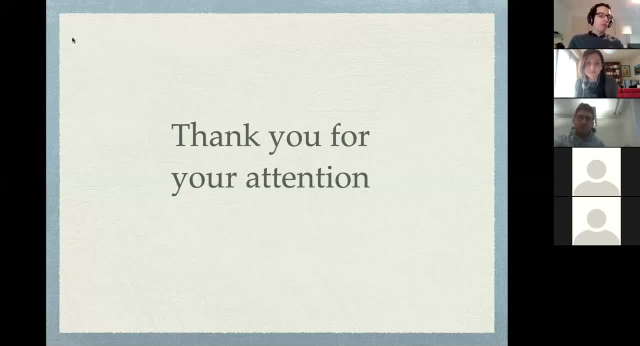 with the afterglow of the GRB than with the external shock emission. So I would like to know if you have an idea if the fact that the environment is very dense has some influence on the origin of this TV emission. The answer is no. 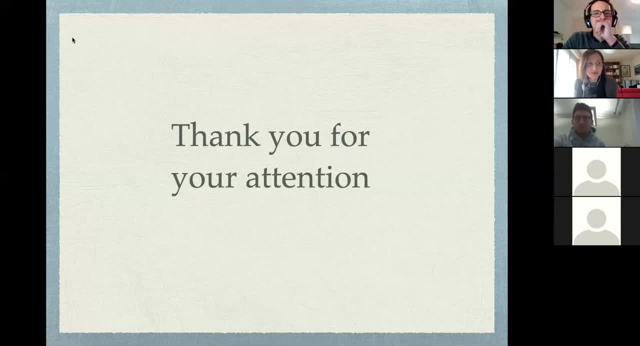 I know that there is this evidence. So we still have a few gamma rebirths detected at TV energies. but this is unusual, unusually large extinction that you see in the optical data, but also the NH from the X-ray. So yeah, I think it's quite interesting. 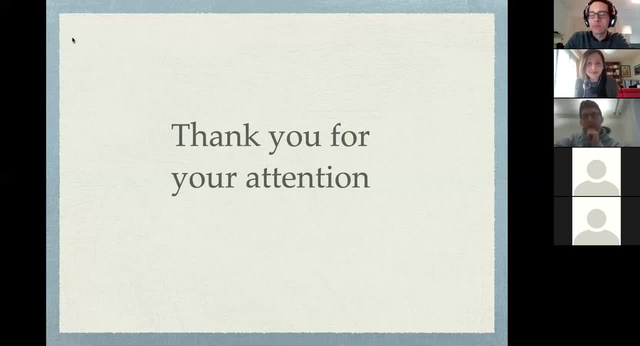 It's not immediate to understand why there should be a connection between this large extinction and TV radiation. The first guess is to have a large density, but I don't know. I still have to think about it. I think that a lot of people 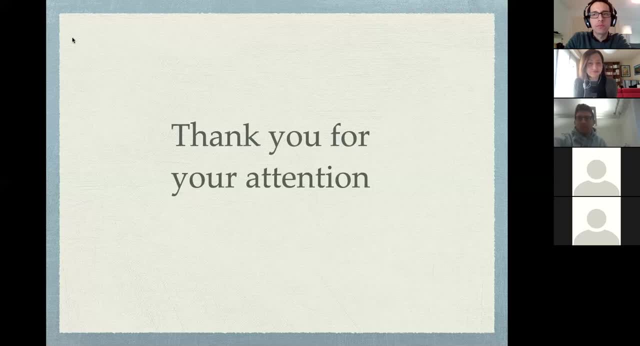 is starting to point out this strange connection. So maybe by investigating more the relation between the density of the medium and the TV radiation, it would be possible to connect the two. Okay, thank you very much. I have one question, if I may. 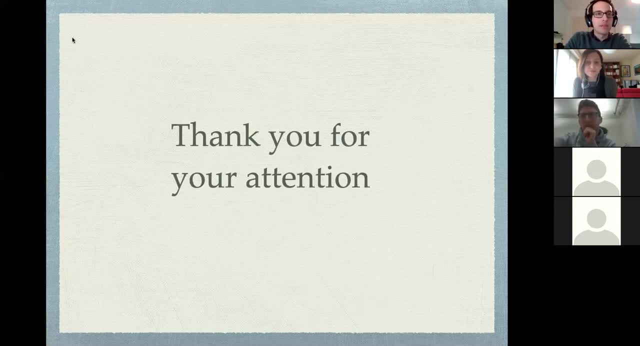 So you're showing that the simple electro-synchronous model sometimes doesn't fit data quite well and you go to SSE and alternatives. My question is: is the statement that the simple synchrotron model doesn't fit the data based on the fact that you have? 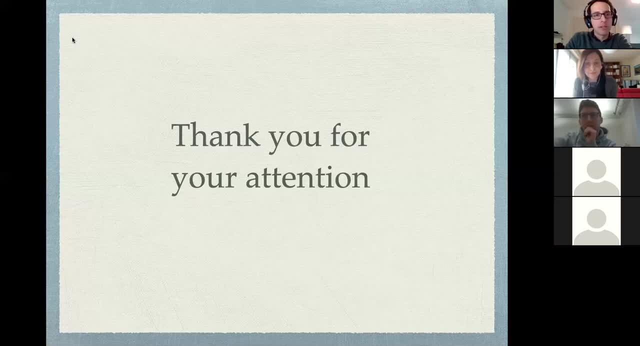 a simple one-zone model where emission and acceleration happen in the same place in the production region. Or is this independent of the one-zone or multiple-zone assumption? No, of course one. So it's very simple, this model. So, yes, one complication that you can add. 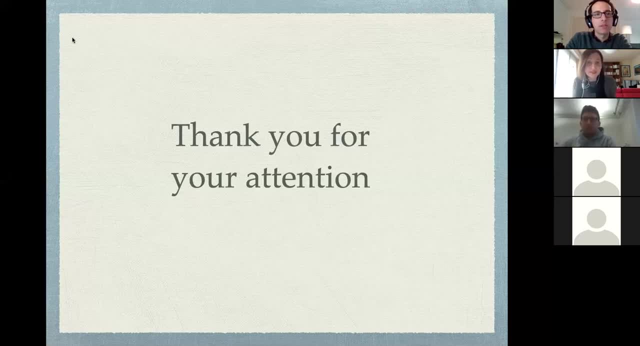 is a devolution of the parameters. Another one is to start to diversify the region where particles are accelerated with the region where the magnetic field, where the particles cool. So, for example, when I show that this epsilon B, that is a parameter that gives an idea. 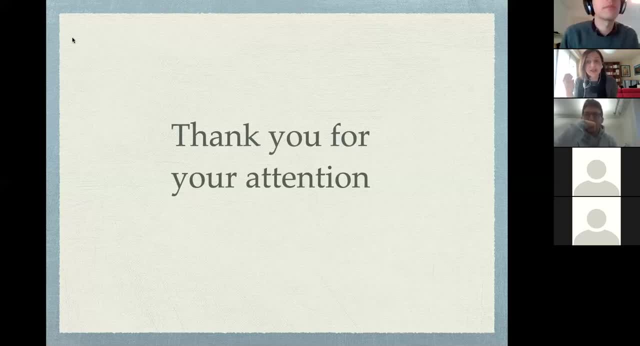 of the amplification of the magnetic field. when I show the plot showing that epsilon B must be quite small, it's unclear: what is this epsilon B? I mean it's the amplification just downstream of the shock, or it's a region where the particle 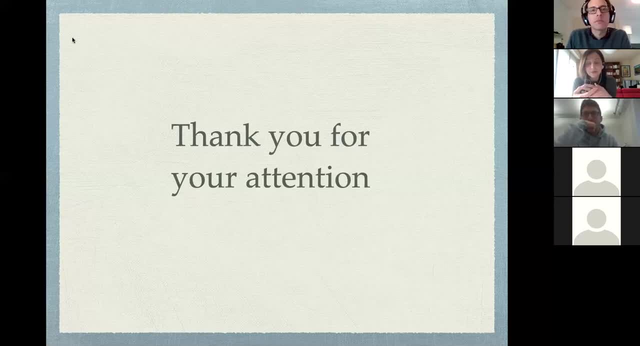 cools more effectively. So epsilon B should be large in order to explain how we can accelerate particles at large energy. We need perturbation in the magnetic field, We need a strong amplification of the magnetic field, But then the question is where the particles really emit most of. 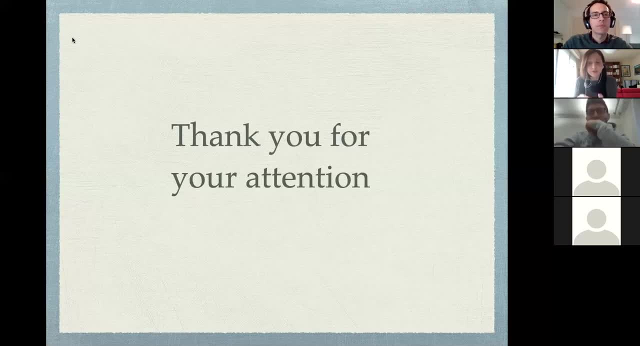 and lose most of their energy. So do they fill this large magnetic field, or the magnetic field decays downstream and the region, the region that we need to invoke for the cooling of the particles- is a region where the magnetic field is already smaller. There are simulations.